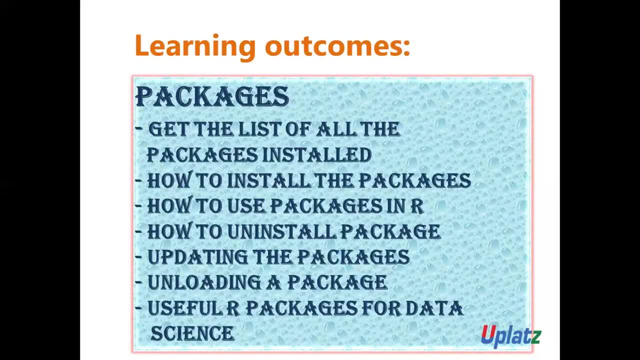 important thing is how to use the package right, And next thing is how to understand how to install the package And then updating the package. how can you update the package And then unloading a package- okay, Unloading the package, And then next thing is useful. 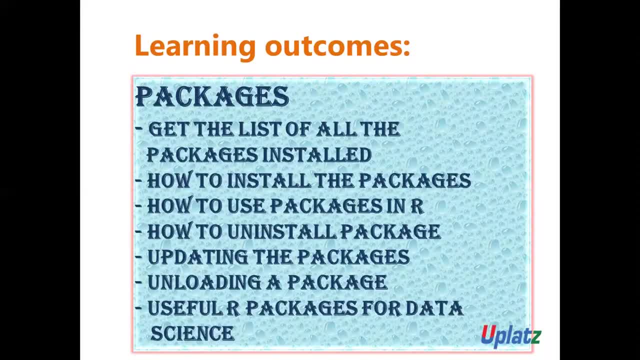 R packages for data science. okay, Useful R packages for data science. So all these topics we are going to cover in this session, okay. So once you understand the package, we are going to see the list of all the packages installed in our R directory. 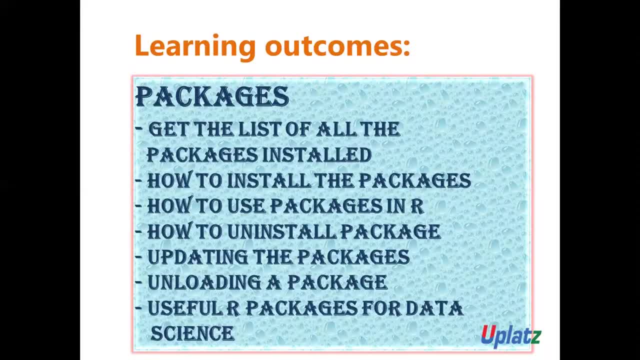 And then how to install a new package, how to use that package, how to load that package And, in case of updation is required, so how to update the package. Let's suppose if you want to uninstall the package, how can you uninstall it, How to unload the package And. 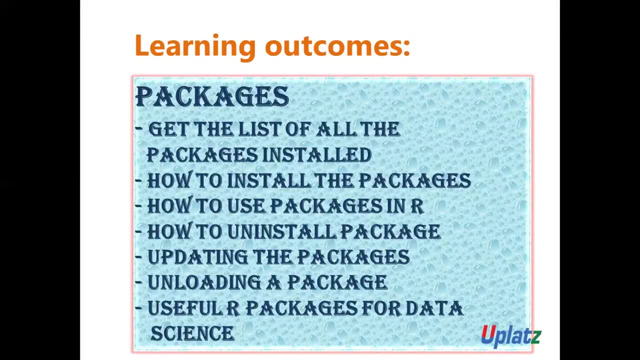 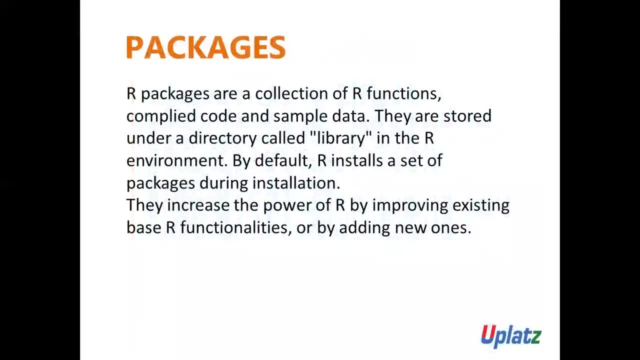 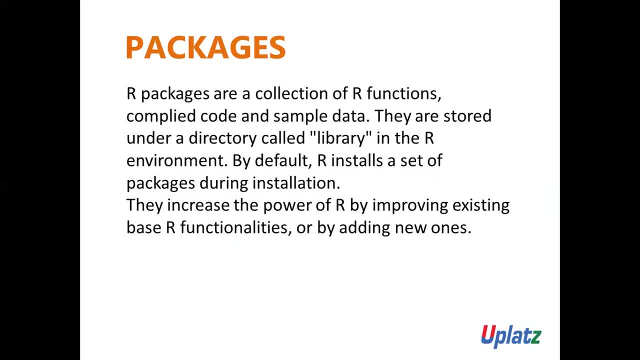 ok where they are stored. they are stored under a directory called library in R environment. by default, R installed a set of packages during installation. ok, that's very good thing for us. by default, R install a set of packages during the installation. they increase the power of R by improving existing base R functionalities or by adding the new codes. 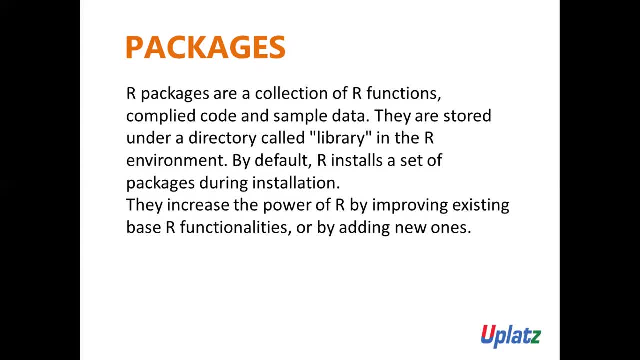 This increases, increase the power of R by improving the existing base R functionalities or by adding the new ones. so you can say: R packages are the collection of the R functions, compile code and sample data, and all the packages are stored under the directory called library in the R environment. ok, and by default R install a set of packages during the installation. 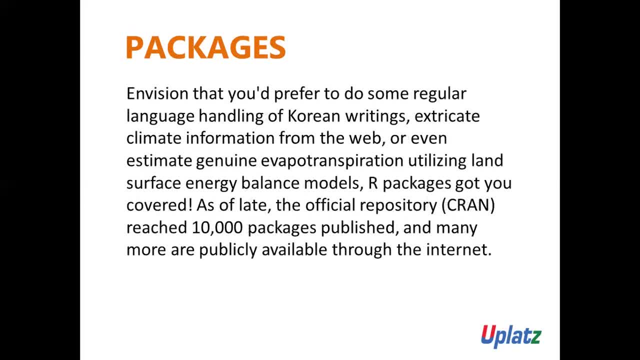 ok. In which, in that, you did prefer to do some regular language handling of a Korean writing. in which, in that, suppose that you did prefer to do some regular language task of Korean writing, ok, or Korean text. extricate climate information from the web or even estimate. 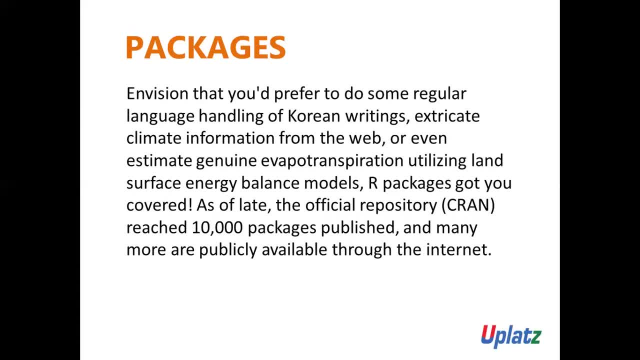 a genuine evapotranspiration utilizing the land surface energy balance model. Ok, or even estimating the genuine evapotranspiration utilizing the land surface energy balance models. R package got you covered as of late. the official repository CRAN. I hope you know that comprehensive RQ network. 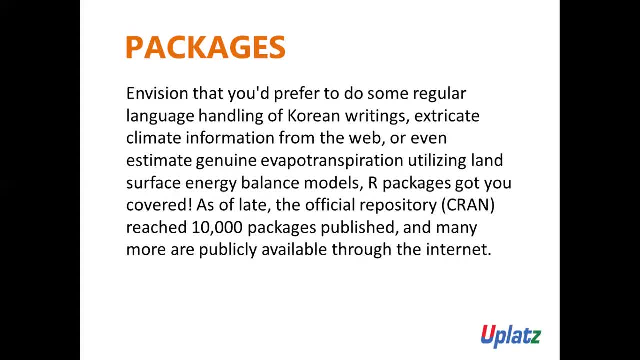 So as of late, the official repository CRAN CRAN reached 10,000 packages published and many more are publicly available through the internet. So, as of late, the official repository CRAN CRAN reached 10,000 packages published and many more are publicly available through the internet. 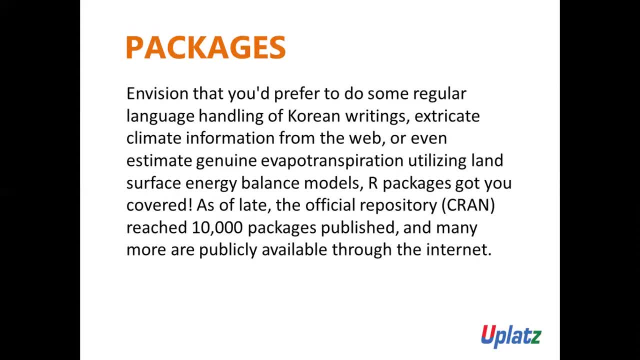 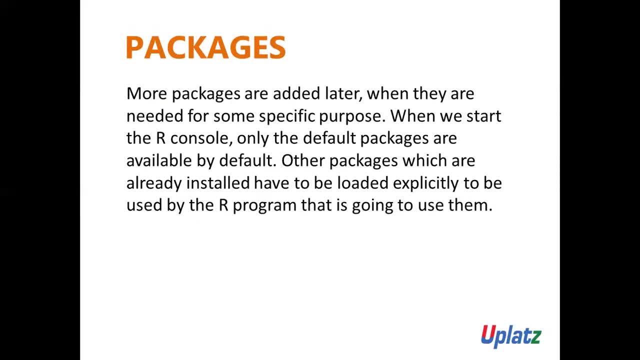 Are you getting it? More packages are added later when they are needed for some specific purpose, so we can add more packages when we need it for some specific purpose. when we start the R console, only the default packages are available by default. Other packages which are already installed had to be loaded explicitly to used by the. 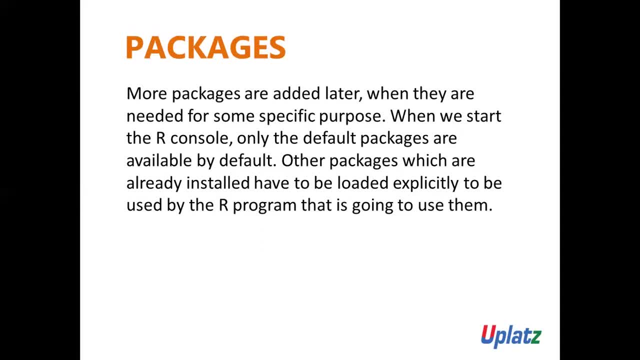 R program that is going to use them, As per the theory, since the R programming language is going to install some packages during the installation. so that package, that all, so some other package which is already installed on your system in RStudio, let's suppose okay. 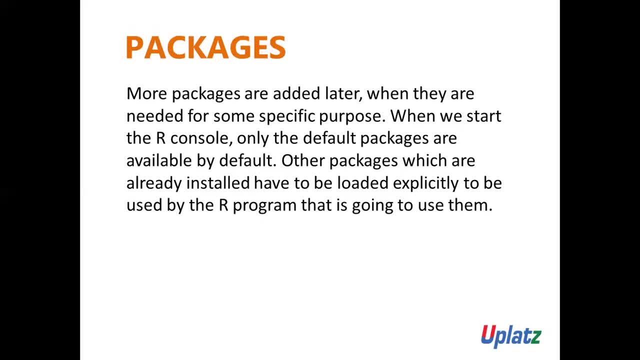 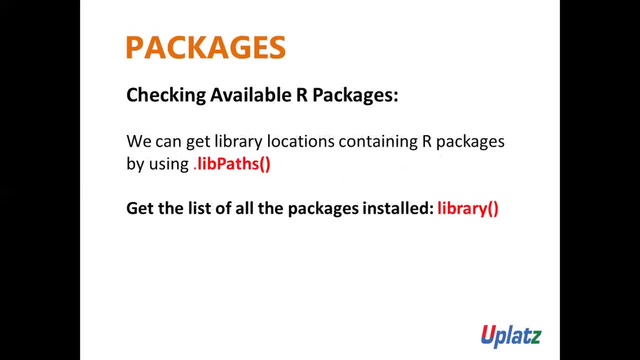 So if you want to use it, so you need to load it explicitly so that you can use it, okay. Okay, now let's see the first thing: checking the available R packages. okay, So first of all, let's suppose, if you want to get a library location containing the R, 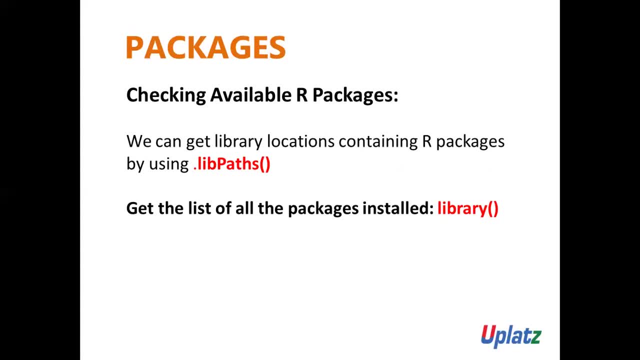 packages. so we can get a library location containing the R packages by using libpath function, See here. as per our theory session, till now R packages are stored in a library Library location, right? So where is this library location? 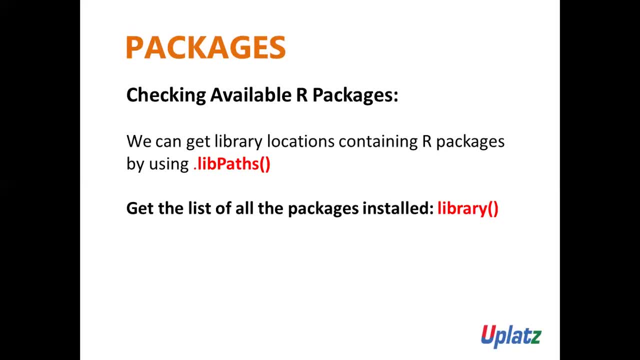 So we can get the library location- library location containing the R packages by using libpaths. this function that I highlighted in red color, okay, And the next, if you want to get a list of all the available package that is installed. 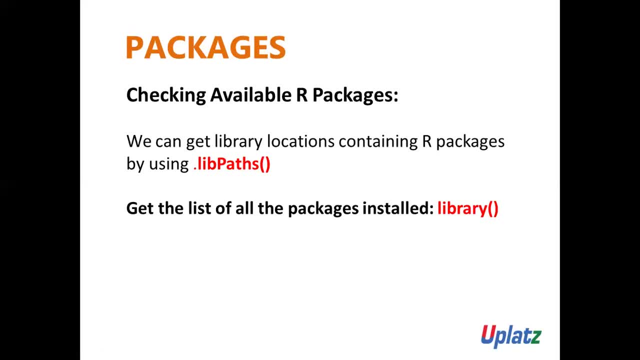 that is already installed in your system in R directory, so you can get a list of all the packages which is installed with the help of the function Library, got it? So library function is help you to check all the available packages. that is already installed. 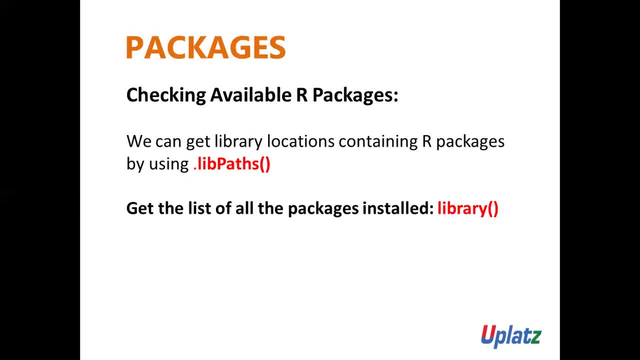 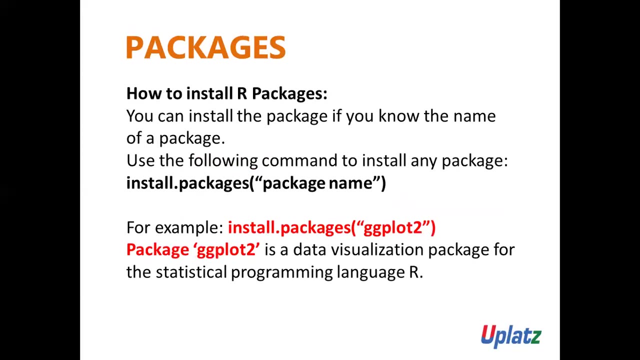 and libpaths function. you are going to use it to get the library location that contain the R packages got it Now next thing is how to install the R package. That's very important. You can install the package if you know the name of the package. 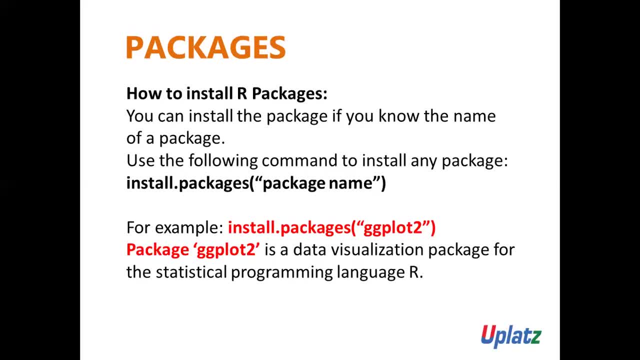 Okay, you can install the package if you know the name of the package. So use the following command to install any package. What is this command? Install that package and then the package name. What is the command here? Install that package. In order to install any package, you need to know the name of that package and then. 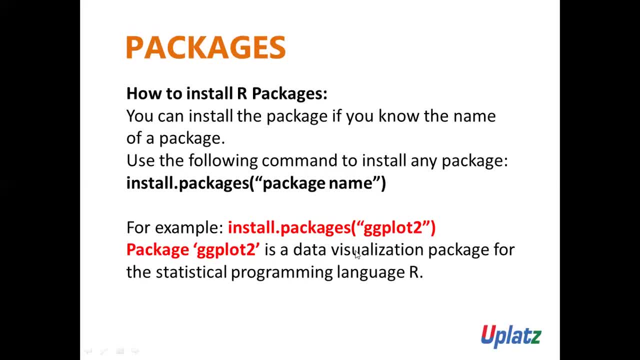 we need to use this command. So, for example, install that packages in double quotation and specify the name of the package. So here, if you write like this: install that package, Okay. inside the opening closing bracket, inside double quotation, you need to specify: 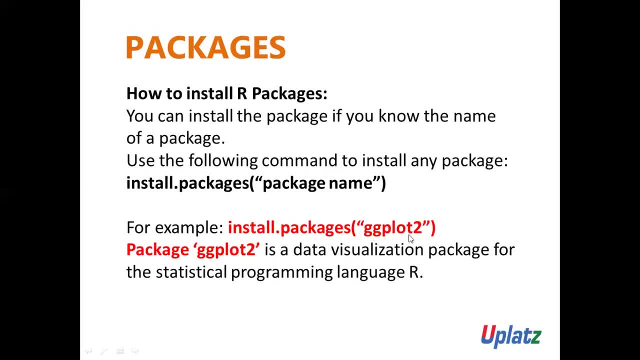 the name of the package. So the package name here ggplot2,. I know that package, So here package ggplot2 is a data visualization package for statistical programming language in R. So ggplot2 is a data visualization package, So I'm installing it. 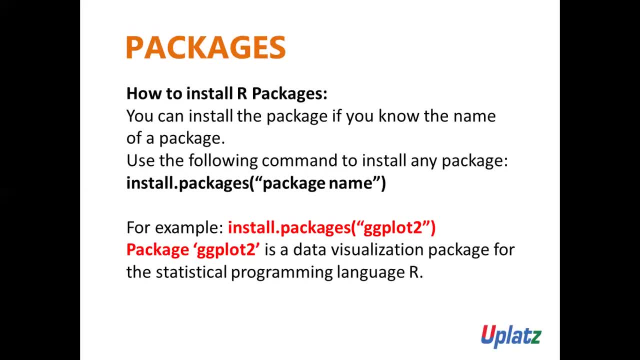 Got it. Now let me show you how can you use this package. So, as per our theory session, once you install the package, Then you need to load it in order to use the package. So let's see how to use the package in R. 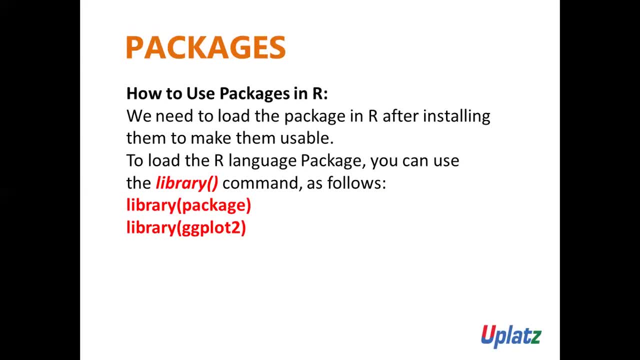 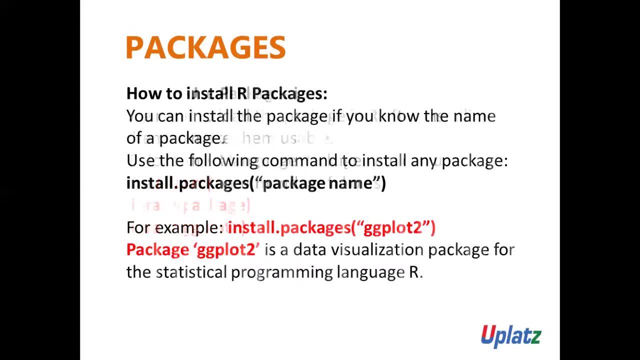 We need to load the package in R after installing them to make them usable. So, once you install the package with the help of function installpackages, With the help of this command, installpackages inside that specify the name of the package. 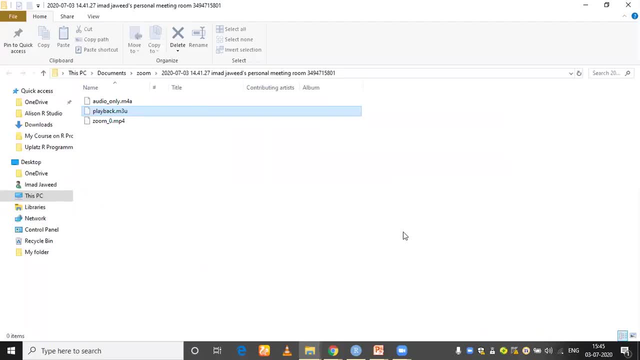 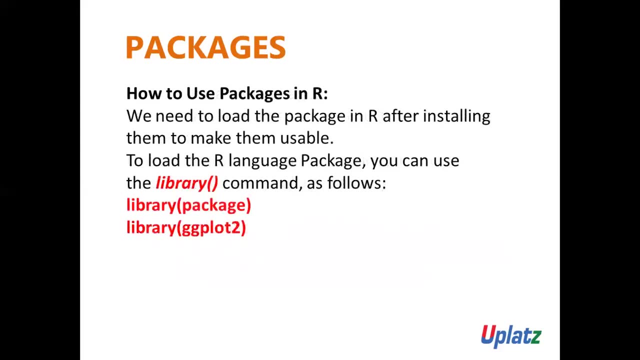 Once you install it successfully, in order to use it. in order to use it, you need to use the function, you need to use the function library. So how to use it? We need to load the package in R after installing them to make them usable. 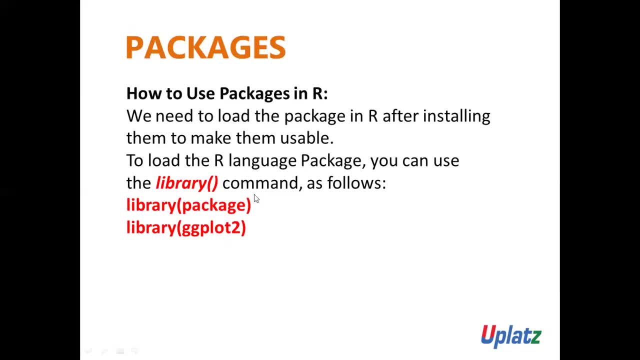 To load the R language package, you need to use the library command as follows, For example, library, and then start okay. inside that you need to specify the name of the package that you installed. So library package name, So library ggplot2.. 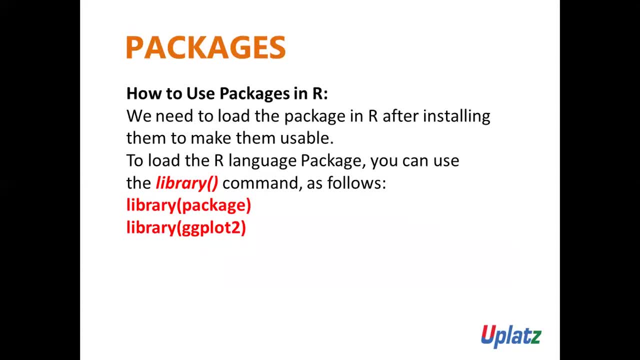 In our previous slide we have installed the package ggplot2.. Now I want to. if I want to use this package, I need to load it with the help of the function library. Inside that library, I need to specify which function, which package, I want to use. 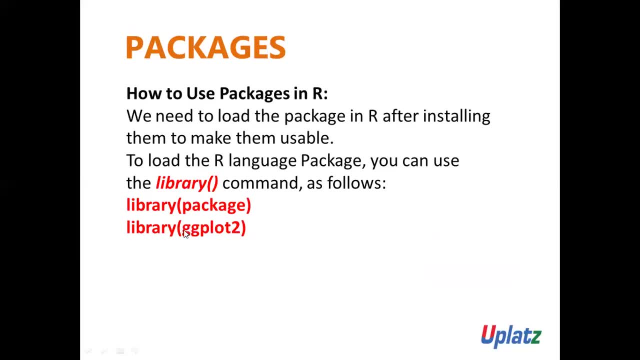 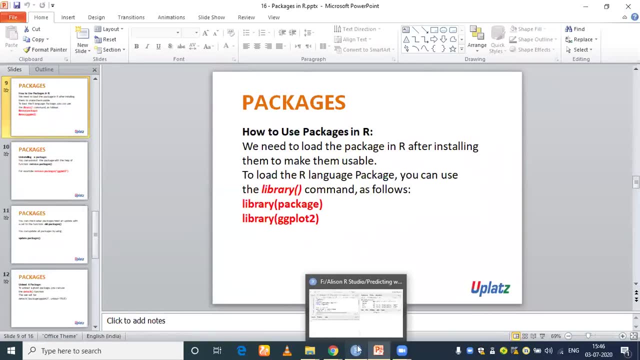 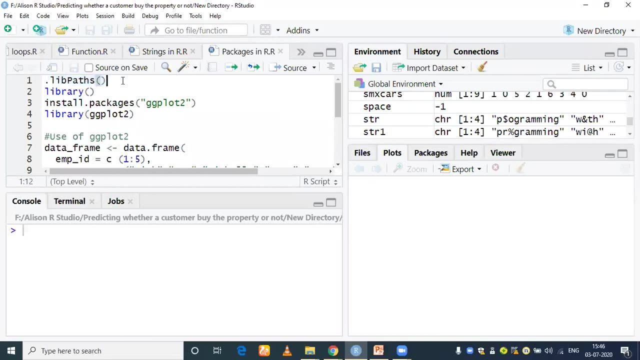 So specify the name of the package that we installed, Got it. Now I want to show you all these things in R studio, So let me open the R studio So see here: libpath. What is that? This? it is going to show us the library location where all the available packages are installed. 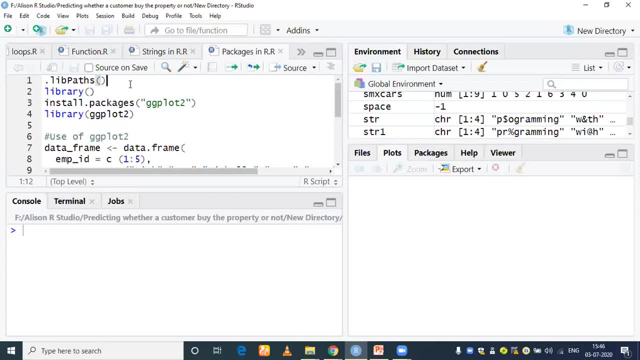 So if I execute line number one, I should get the library location. So see here, this is my current library location, where all the available packages are there. Can you see this? one, One and two. Okay, Now next thing is library. 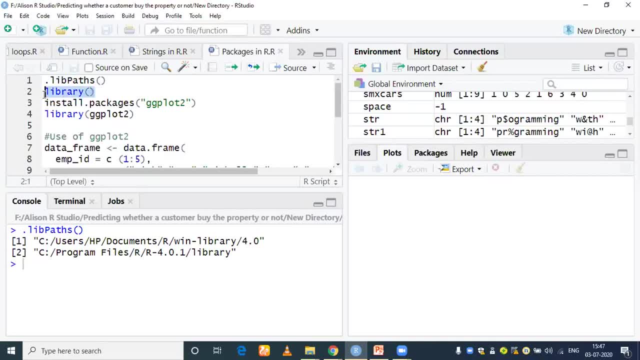 If you just write library function like this: If you execute this, you are going to get a set of all the available packages that is currently installed, a set of all the available packages that has been installed. So if I execute line number two, I should get all the available packages. that has been. 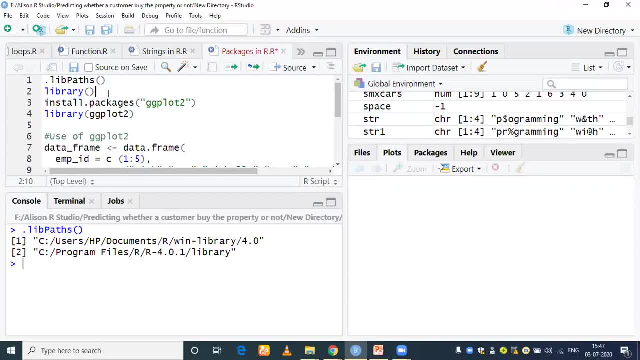 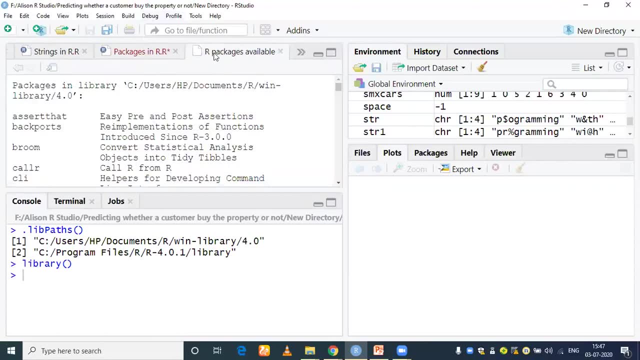 installed. Okay, So let me execute line number two. So I have executed line number two, So see, here it's running. Can you see a new tab has opened. now R package available. Can you see that Packages in a library? which library? 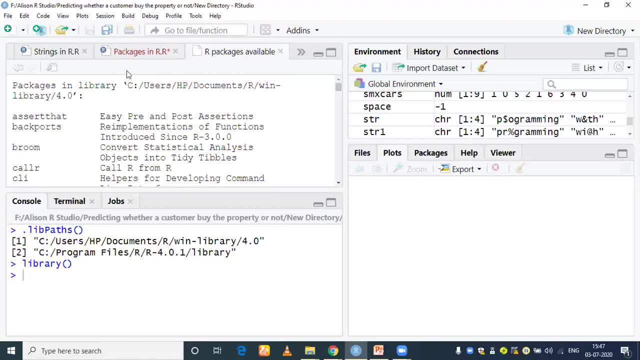 Since the packages are stored in a library. So first of all, with the help of the function libpath, we have find the library location. So this is our library location. See here: see user HV, document R. we'll see here this one. 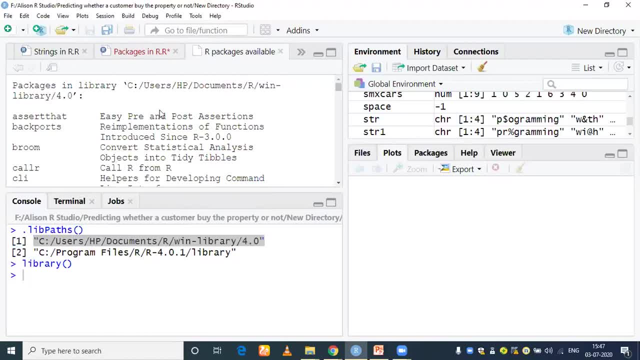 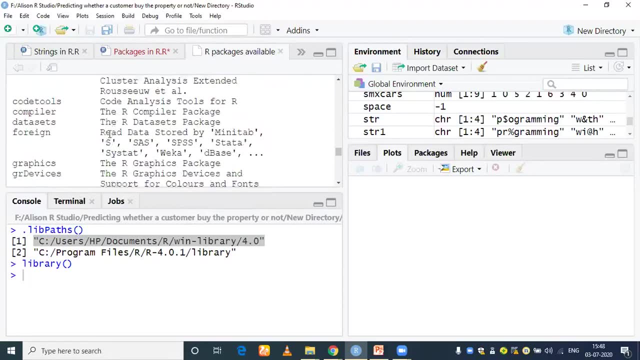 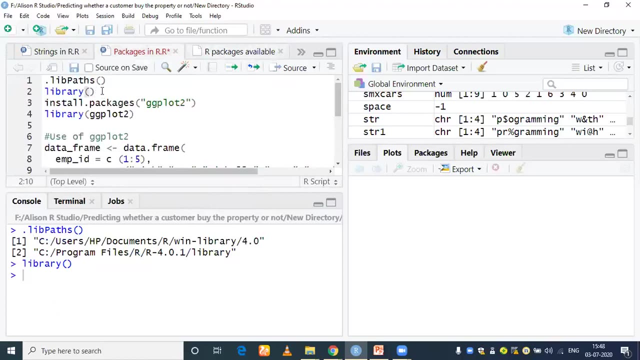 Okay, So in this library part, in this part, which packages are available? See here: all these packages are available. Can you see this one? Yeah, Got it. So with the help of this function, we can see all the available packages installed in. 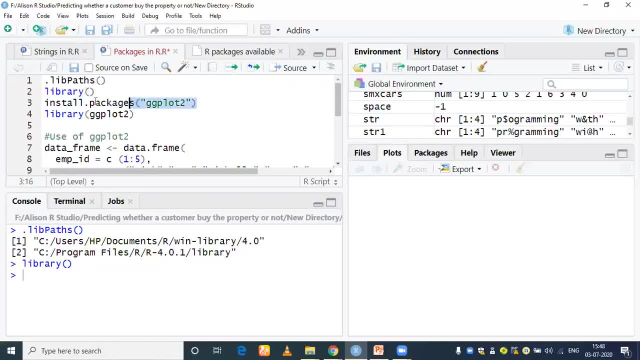 our system. that is installed in our system. Now let's see focus on line number three. If you want to install a new package, you need to know the name of the package. So I know the name of the package, that is, ggplot2.. 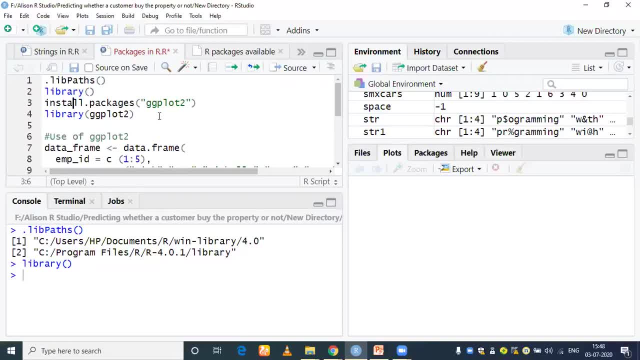 That is very important for a data visualization. Okay, ggplot2 play a very important role for a data visualization. This is one of the most important package, So how can I use it with the help of this command Installpackage? I need to specify the name of the package if I double code. 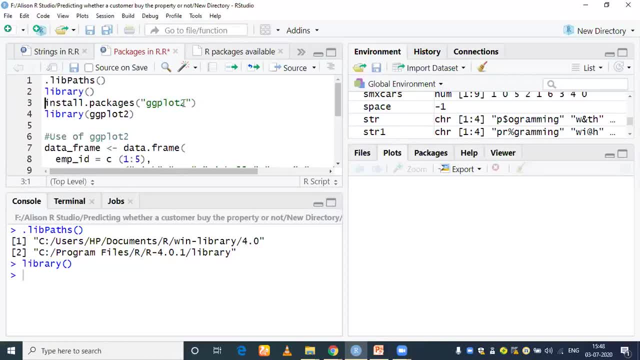 So if I execute line number three, it is going to install the package ggplot2.. So let me execute line number three. So see here line number three. it is started for execution, So wait for it. Okay, What's happening? 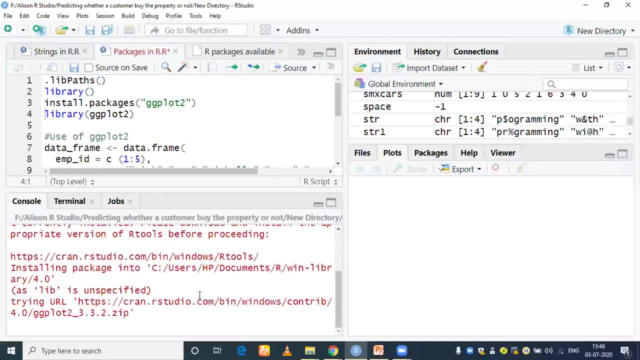 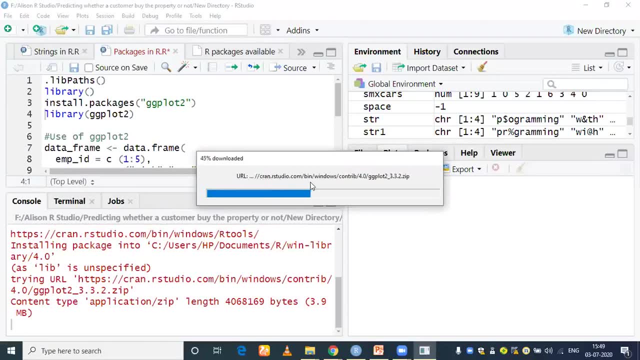 It's just giving the warning, So let's wait. What? what happened? Let's read it. So can you see that it's started to download, Yeah, From the website. So I hope now, yeah, with the help of the command installpackages. you just need to. 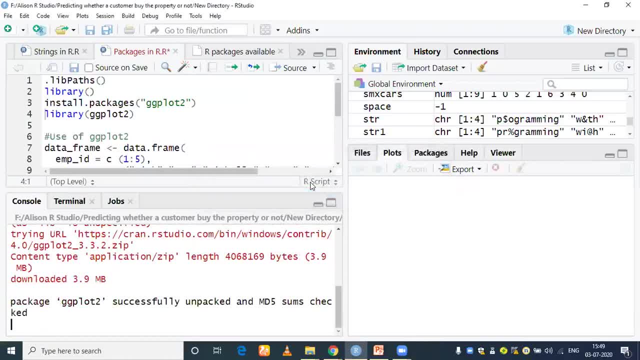 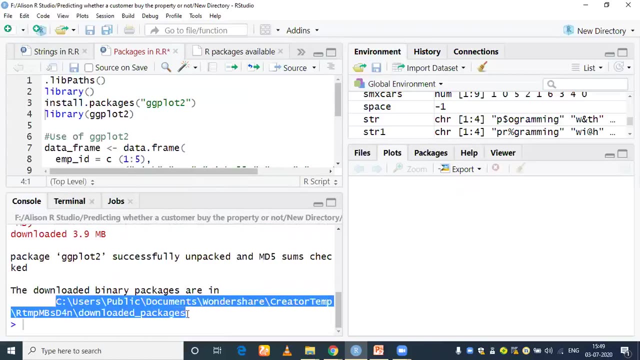 specify the name of the package that you want to install And finally it is going to install. So can you see on the console screen: package ggplot2 successfully unpacked and MD sums checked. So see here. it is also showing you the download. binary packages are in this directory. 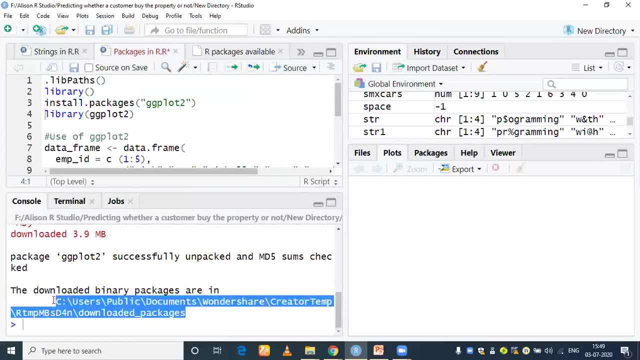 Okay, This part It's installed in. this part Got it. So with the help of this command, we can easily install the package If you know that package name. now, in order to use the package- as far as theory you know, to use the package that you install- you need to load them with the help of the function library. 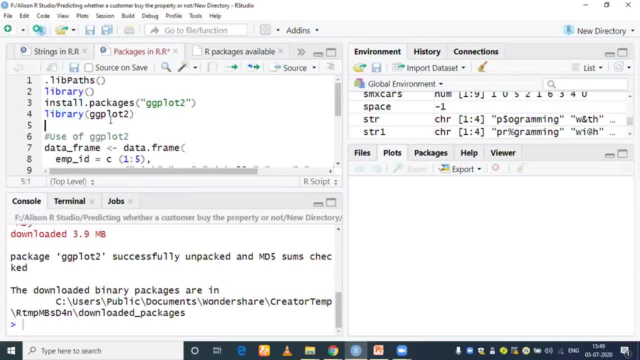 So I'm using the function library Instead that you specify what package you want to use. So if you just write library, like That I highlighted on line number two, you are going to see. you can see all the available packages. Okay, 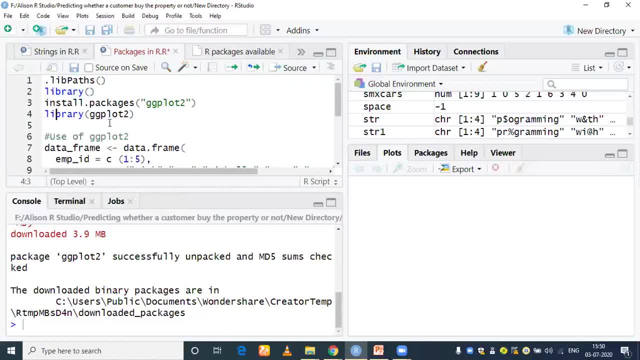 But in order to use a specific package- okay, That is installed in your system, You need to load it with the help of function library. inside that increase, specify the package name that you want to use, So You simply be installed: the ggplot2 package. 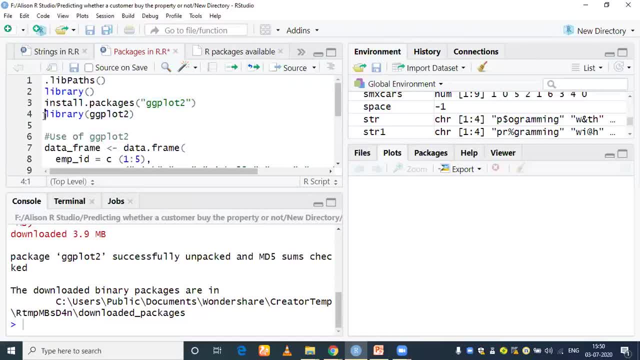 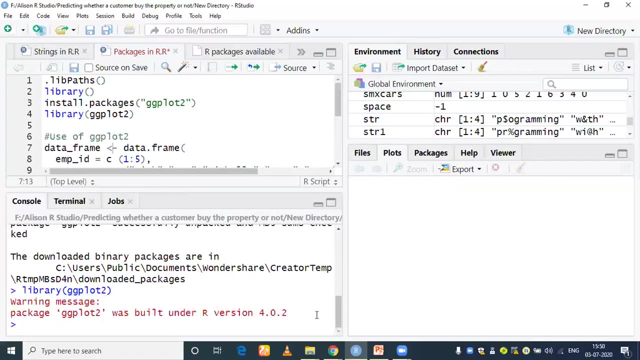 Obviously you want to use it, So let me use it. So I will execute line number four. So see line number four. I have executed successfully. Now I can use the ggplot. So see here it's a warning message. It's a package. ggplot2 was built under our version 4.0.2.. 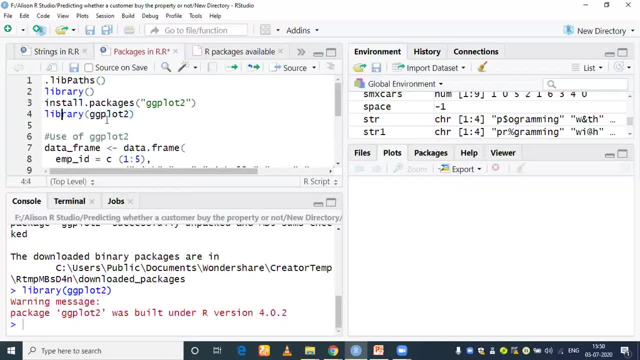 Okay, It's okay. So this means now we can use the package ggplot2.. Okay, Now let me show you how can you use it. So, before going to show you this ggplot, okay, As I told you, it's one of the important package for data visualization. 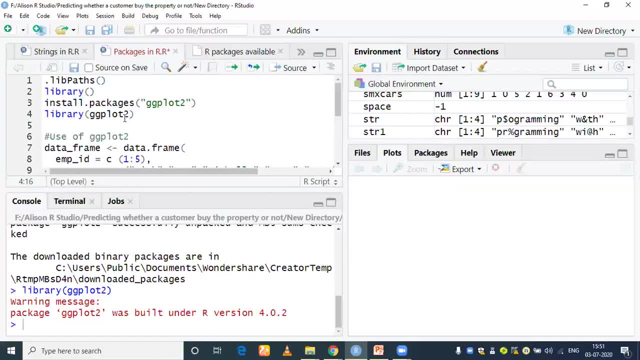 Okay, Through which you can draw the plot. Okay, Are you a scatterplot or whatever? it is Okay And, by the way, we are going to see the various types of graphics and the plots supported in our programming, such as boxplot, barplot, histogram, scatterplot. 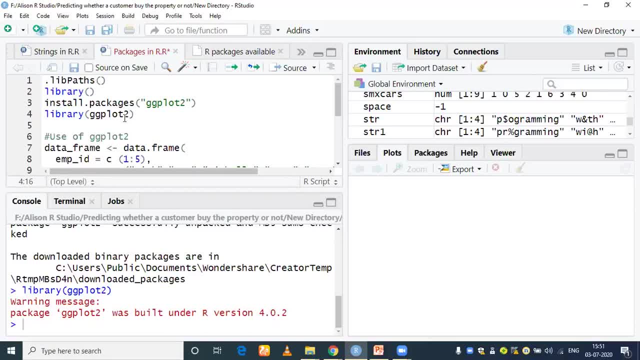 Okay, And then any other type of plot supported in our in our later sessions. But here, as we have installed the package ggplot2, as we load it, I just want to show you a basic, basic thing about it: how to use this one. 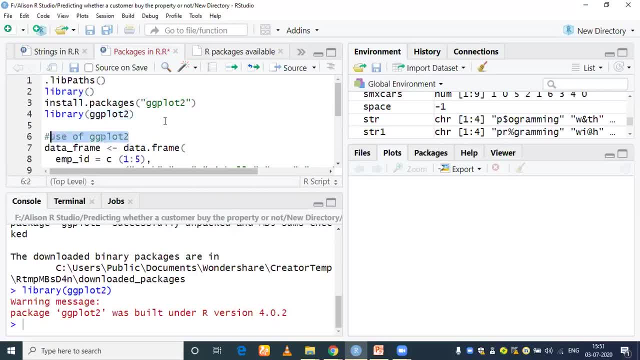 Now, before going to use this one Use of ggplot2, I want you to create a data frame. I hope you remember how can you create a data frame with the help of function dataframe. you can create a data frame, am I right? 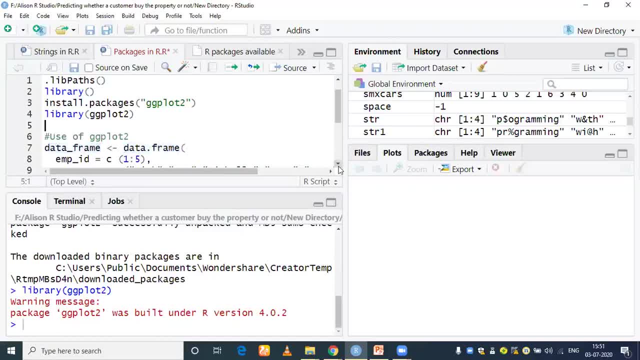 And I'm assigning a name to it: data underscore frame. So how can you create a data frame? So, employee ID: that is a name of first column that contain the five observations. one colon: five. This means five rows. Employee name: again the name of the column. 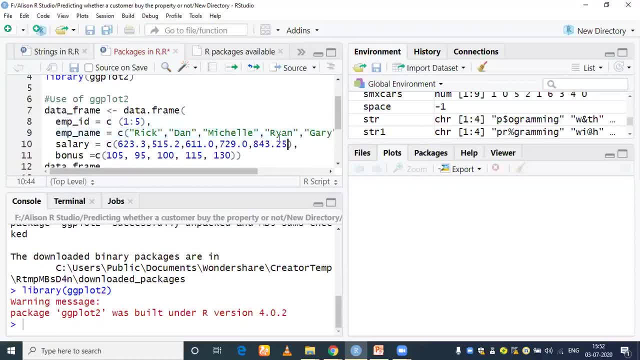 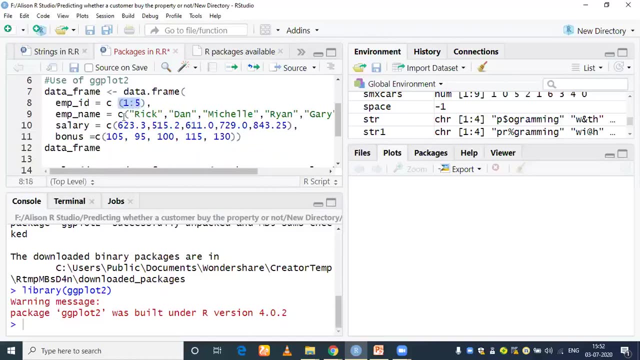 Okay. Second column that contain this observation: These rows, Okay. And then the salary. again a third column name. bonus is the fourth column name: Okay, So see here. each of the columns should contain equal number of observations. So, employee ID: contain five observation. employee name should also contain five observations. 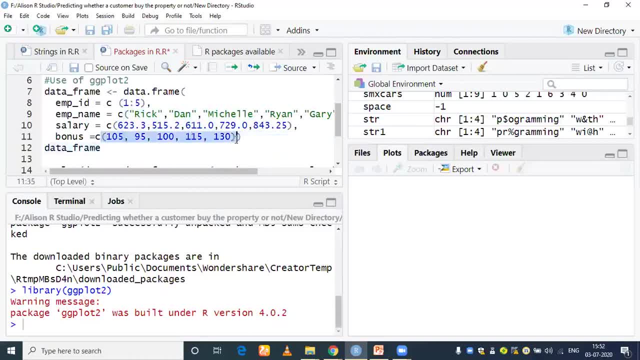 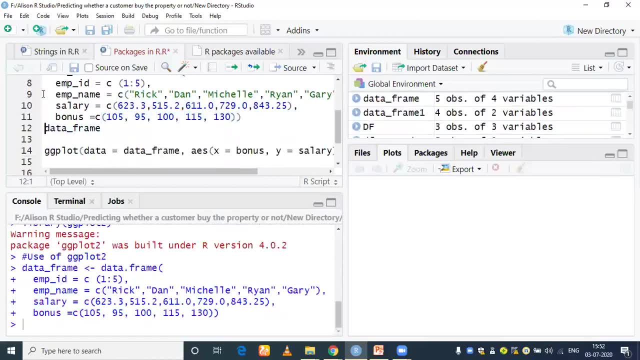 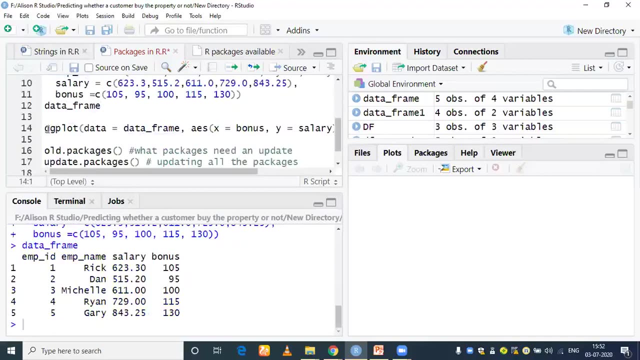 Salary should also contain five observation. bonus also contain five observation. After that, we need to close it. So let me execute line number seven. So see data frame. data underscore frame has created. Now let's see the output of it. I will execute line number 12.. 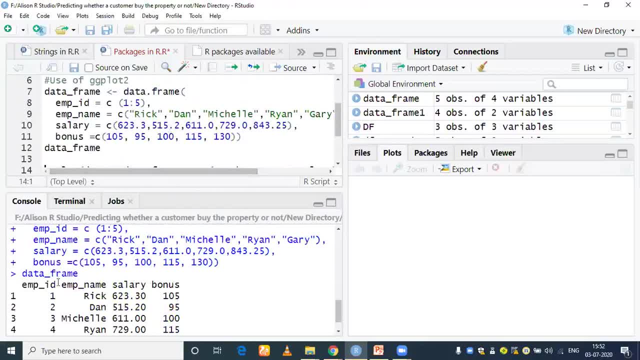 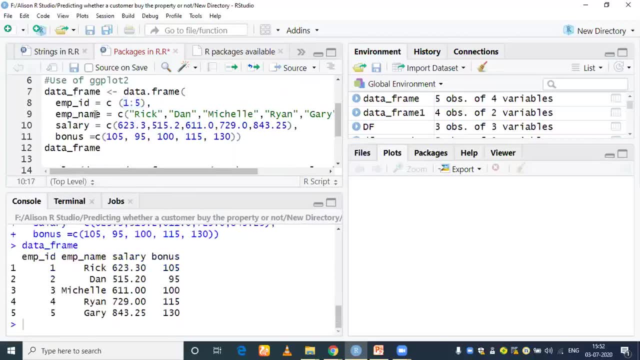 So see here data underscore frame. So what is the name of first column? we have given Employee ID. one colon five. So one, two, three, four, five. Next column name is employee name, whatever we specified here: Rick, Dan Michael and. 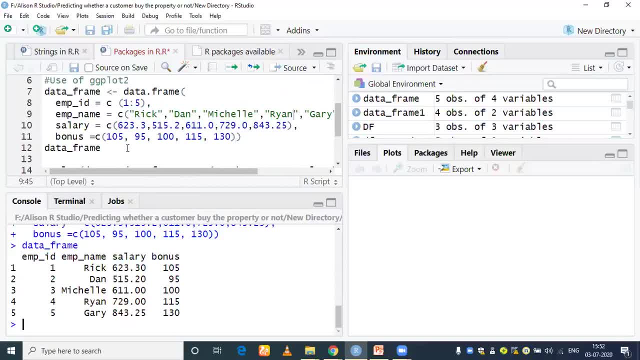 then the salary, Okay, And then the bonus. So, in short, you can say: we have created a data frame with five columns, with four columns and five observation Okay, Or five rows, But it now I want to use this function, ggplot2.. 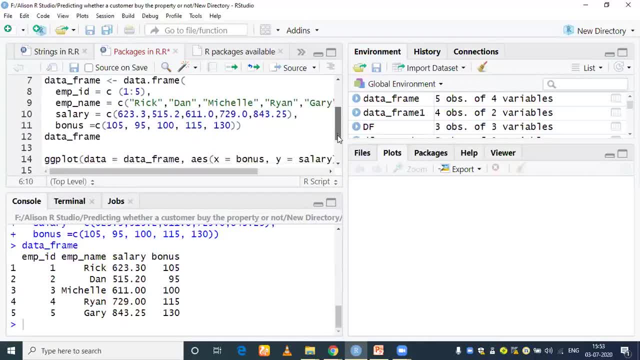 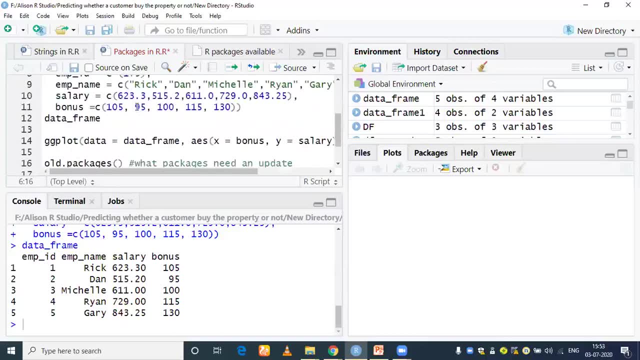 I want to use this package, So let me tell you how can you use it. You need to write ggplot. Okay, This function Don't write ggplot2.. ggplot2 is the name of the package, So ggplot, write, write, ggplot function. inside that write data is equal to what? 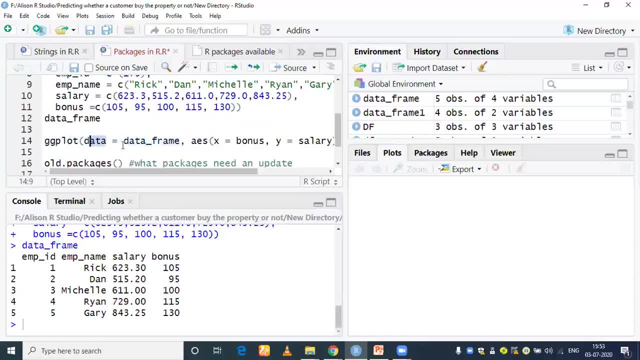 What data you want to use for ggplot. So write data is equal to what is the data we want to use here, The data which is available inside the data frame. So what is the name of the data frame here? Data underscore frame. 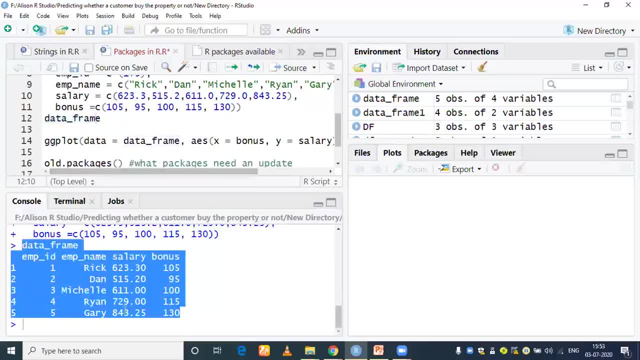 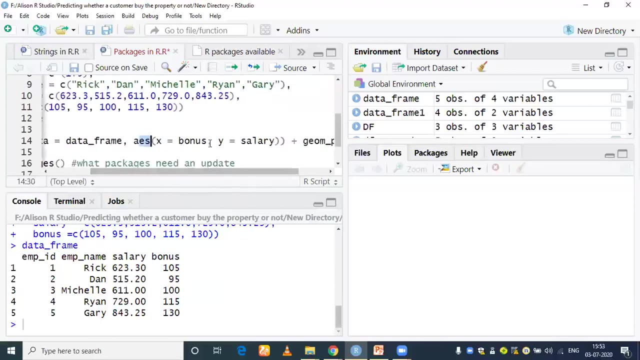 So see here, this is our data underscore frame. I want to use this data. Okay, To plot. Okay, So I will use. data is equal to data underscore frame. This data: Okay. After that, AES means aesthetics, in which you are specifying what you want to have on. 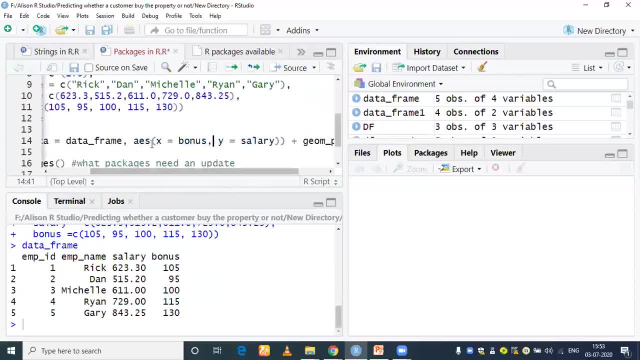 X axis and what you want to have on Y axis. So I want to have bonus, this data, bonus data on X axis and salary data on Y axis. So hence I return aesthetic of X like this, focus on this line. aesthetics X is equal to. 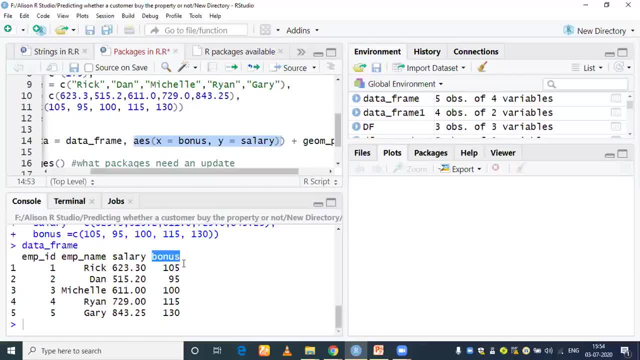 bonus. This means an X axis. I can see the data about the bonus. one zero five, 95 is a hundred, and on the Y axis I can see the data about salary. So see the salary And finally you need to close it. ggplot data is equal to. 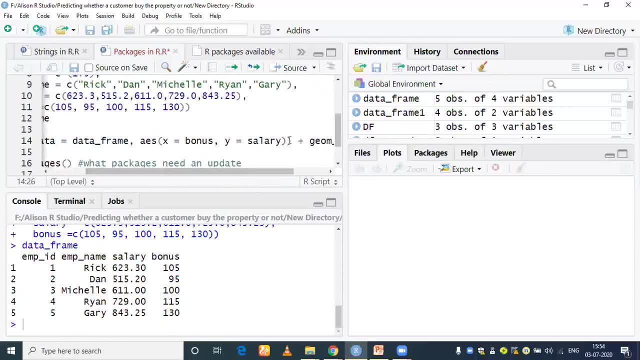 Data frame, comma aesthetic is equal to this one. And then you need to close ggplot two. Okay, So ggplot function And after that you need to write geom point. This means you want to highlight this plot with the alpha point, g, e, o, m underscore point. 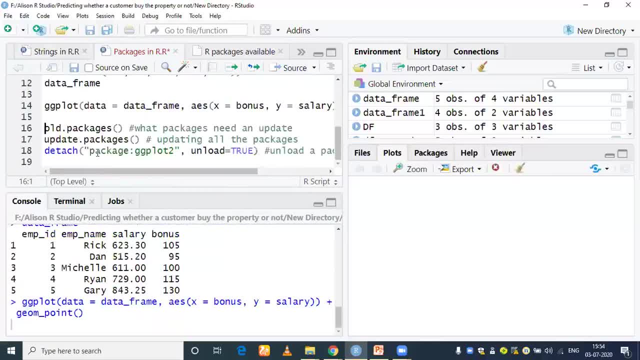 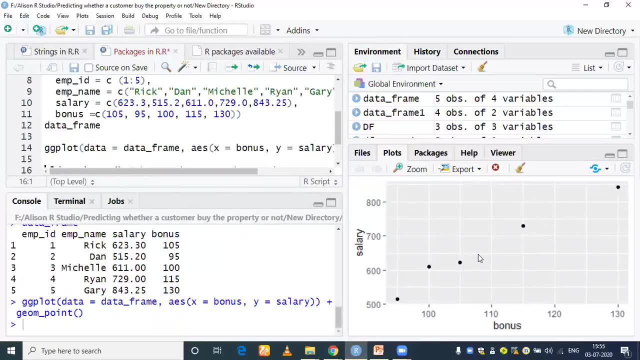 So let me execute now line number 14.. Now, wait a minute. Can you see the output here? Can you see the plot here? Yes, Okay, So we have draw a plot. Yes, Can you see that with the help of ggplot? 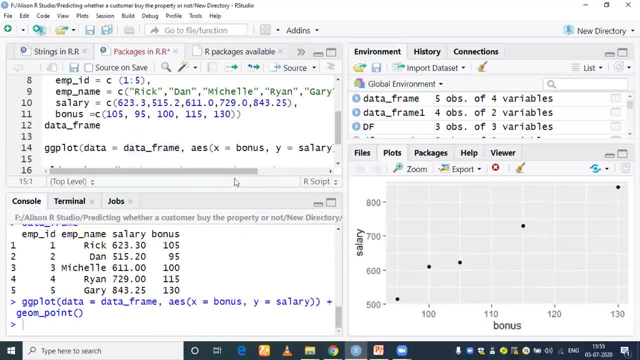 So, in which we have used the data for a data frame on which we have used aesthetic, X for a bonus, So see here the bonus and Y for the salary. Can you see that bonus on the X axis, Y and salary on the Y axis? 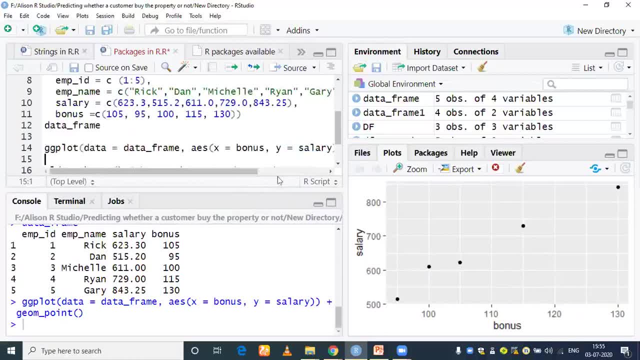 Okay, And then the geom point. So whenever the data is matching the corresponding data. So see here. Can you see here? Okay, So geom point. So it is going to represent our plot with the help of point. Can you see that? 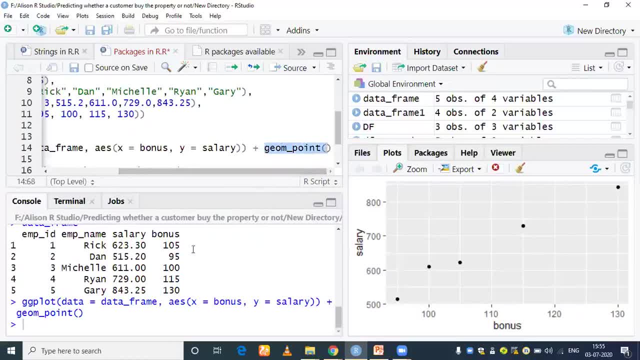 Now, if you focus here, what is that? 95,? 95 is belong to five and five. So see here: 95 is belong to five and five. The first point got it. now, in case of a hundred, can you see this: a hundred, a hundred belong. 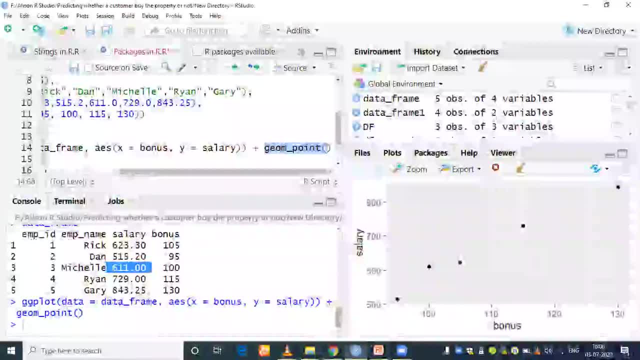 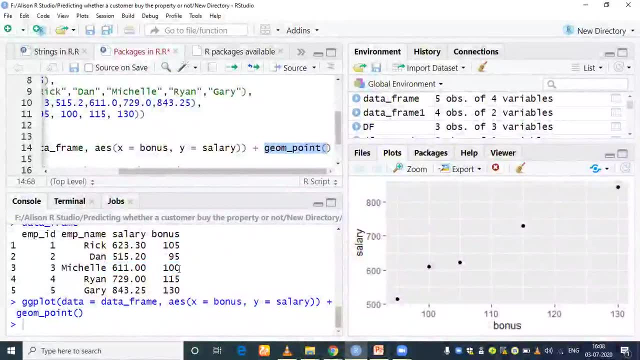 to six, six, one, one. Can you see this one? A hundred belongs to 80.. Can you see this one? If the value of bonus hundred, okay, the salary is six, one one. See here. So if the bonus that we have plotted on the X axis, the value for, is hundred and the corresponding 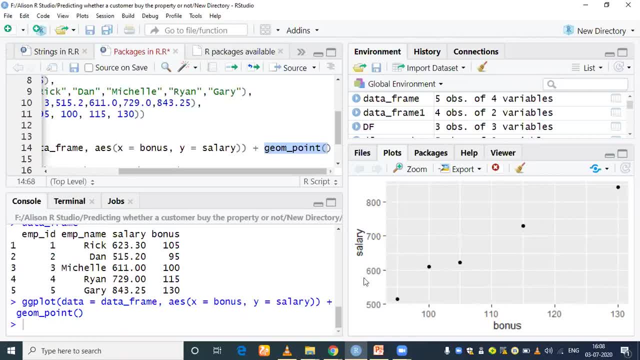 value for a salary that we have plotted on the Y axis is six one one. So see here: six one one. And then next, if you think about what is this: one zero five, one zero five. if the bonus value is one zero five, the salary value is 623. 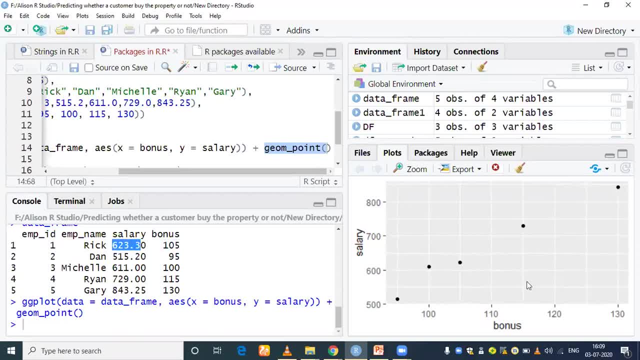 So see here, And what is this? It's look like a big one. Yeah, One one five. So if the bonus is one one five, the salary is 722.. See here, got it. See here. 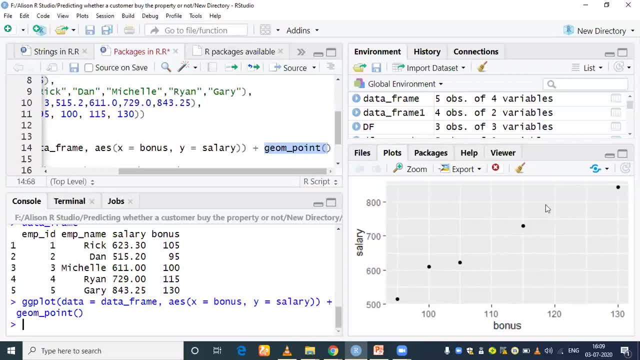 And then last one: if the bonus is one 30 salaries, 843,. can you see this last one? Yeah, So I hope you got it How we have created a data frame, Okay. So, by the way, we have created a data frame so that we can use the data to plot. 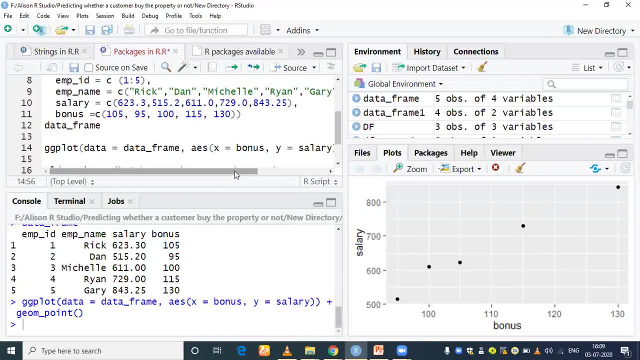 Okay, To make a plot with the help of ggplot function, So I hope you understand how to use it. inside a ggplot function, to write data is equal to name of the data that you want to use, data frame And then specify aesthetics, AES. this function contains X is equal to bonus. 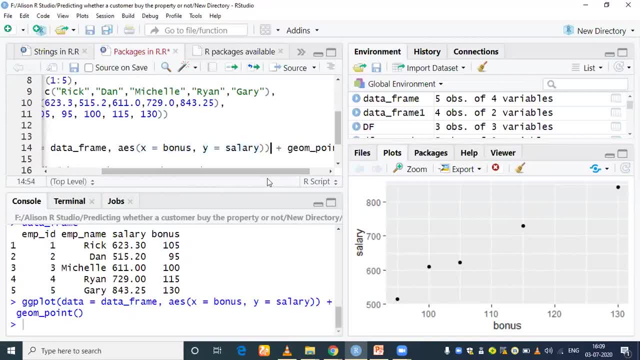 What do you want to plot on X axis and what do you want to plot on Y axis and close the ggplot function And then after that you write geom underscore point so that the point can be plotted. Can you see that? But if you write geom underscore line also. so let me show you what occurred, what going. 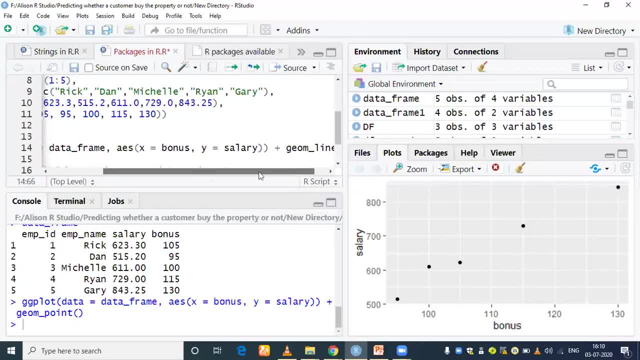 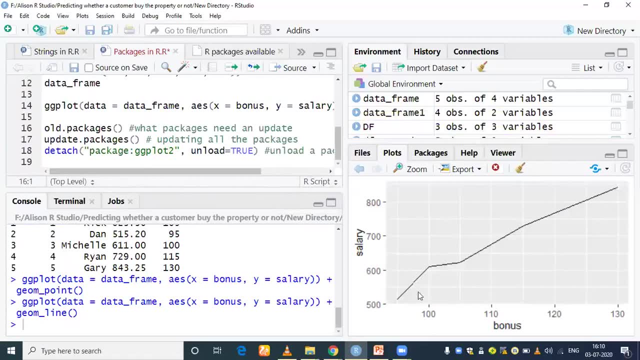 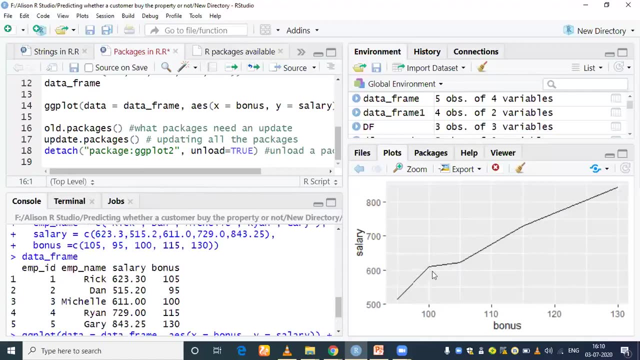 to happen if you write like this: one geom underscore line. So initially it's the plot. Now, if I execute line number 14, so see here, can you see that? the first point, the second point, third point, fourth point, five point, because we have the data with five observations. 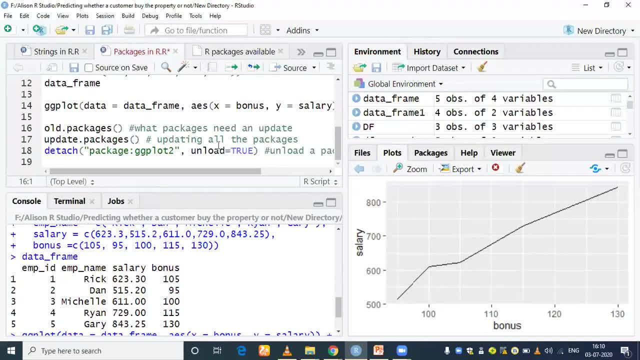 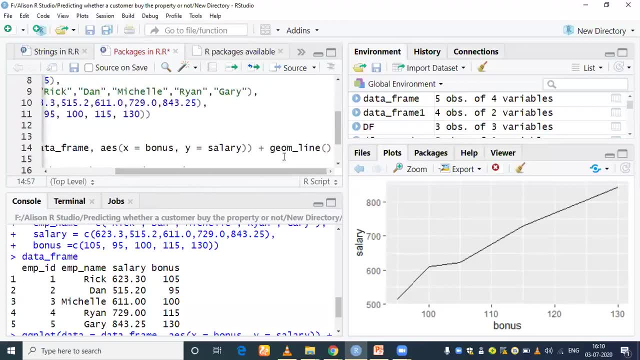 Can you see that? But even if you want to write in, if you want to make it more, uh, what do we say? If you want to have this plot look like more good, Okay, So I what I will do. I will add geom point also, plus geom line. 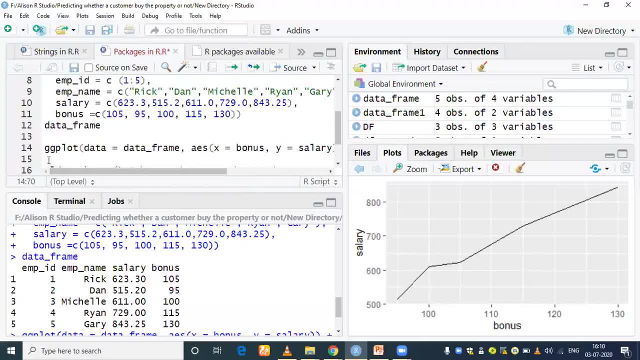 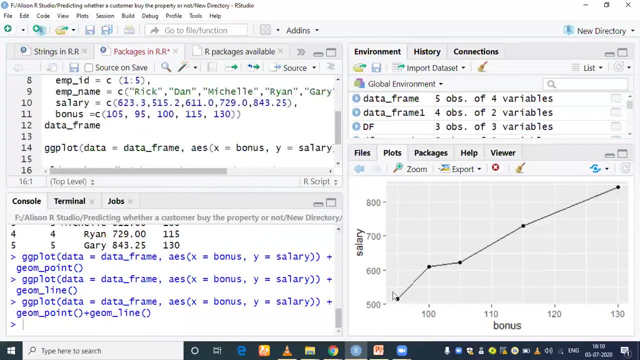 What I have done: geom point plus geom line. So let me execute lies Now. can you see that we have plotted a plot that contain the plot? Can you see that? Can you see that? Okay, So this is the point, as well as the line. 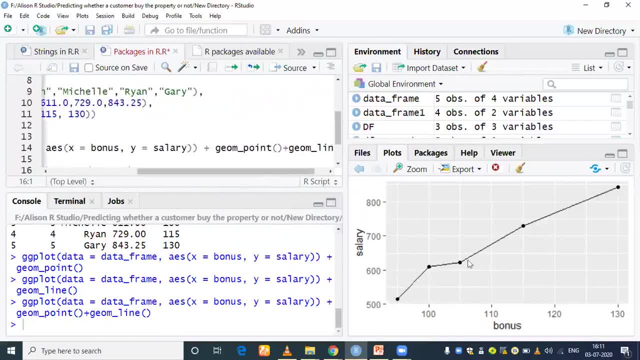 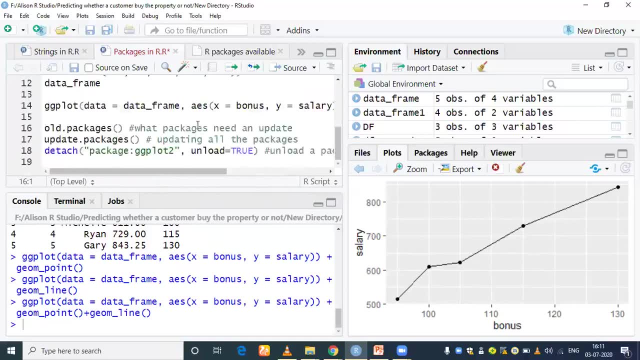 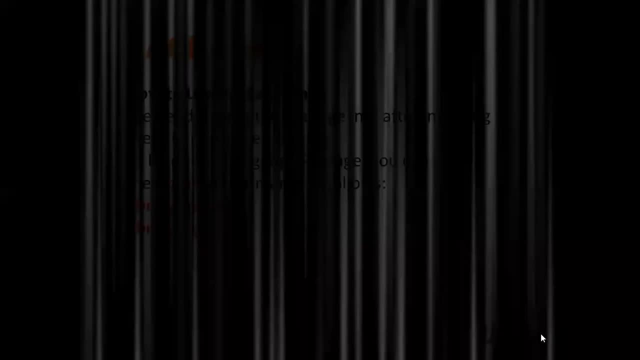 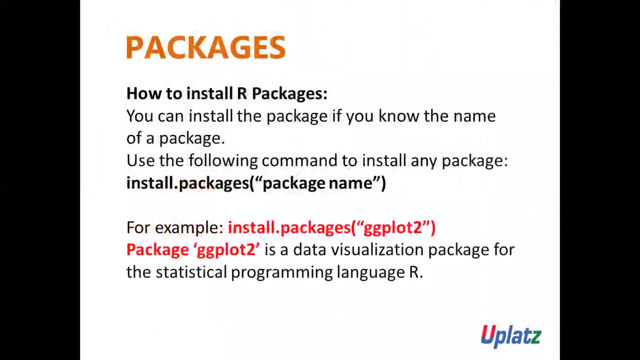 So this point is nothing but this one geom point and geom line that is connecting with each point with other one. Yeah, So what it? so I hope you understand now. now let's see next topic about packages. So till now we have seen: yeah, with the help of lib paths you can see the library location. 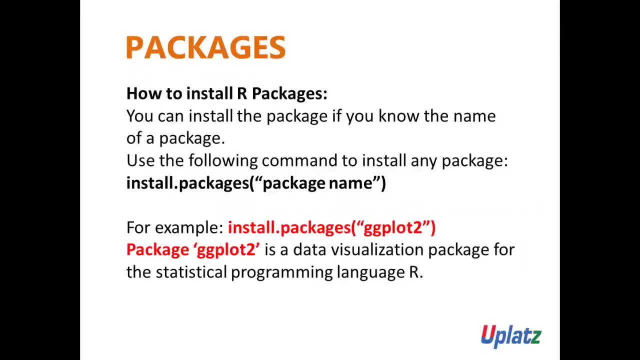 where the packages is installed. After that, we have seen the library function, through which you can see all the available packages. Okay, And after that, in order to install the R package, we need to use the command installed R packages And inside that we need to specify the package name. 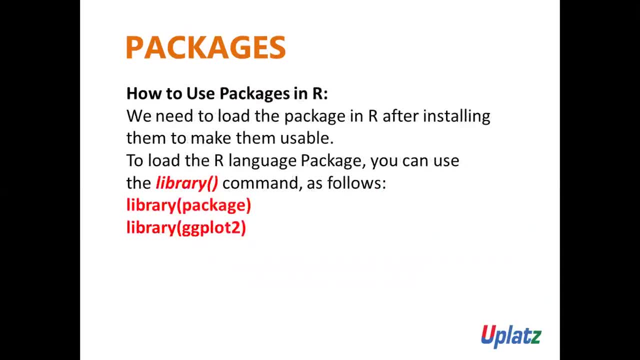 Once you install the package successfully, in order to use that package you need to use the, you need to load it with the help of function library and inside that library function, you need to specify the name of the package that you want to use. 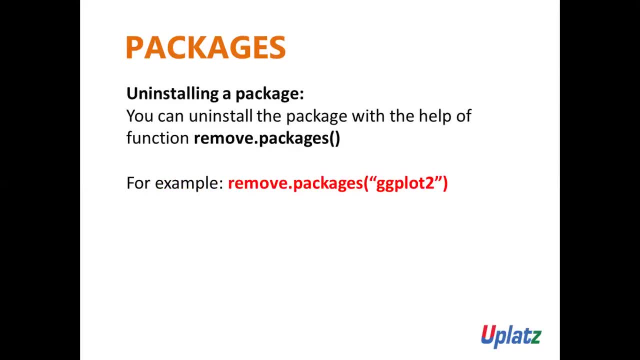 Okay, Now let's see how to uninstall a package. Okay, You can uninstall the package with the help of the function removepackages. okay, So can you see this example, removepackages- and then specify the package name that you. 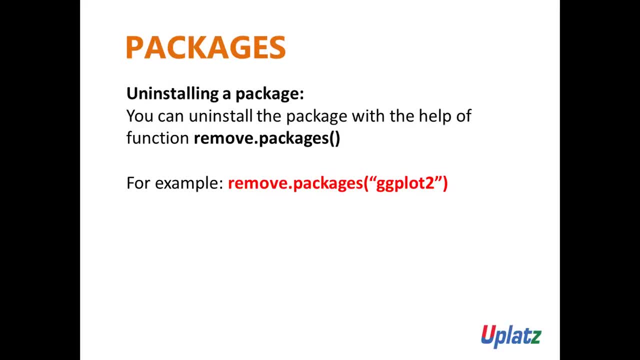 want to uninstall, So removepackages. So recently we have installed ggplot2 package. okay, We have loaded to use it and we have used it to draw the plot. Yeah, After that? now let's suppose if you want to remove it. 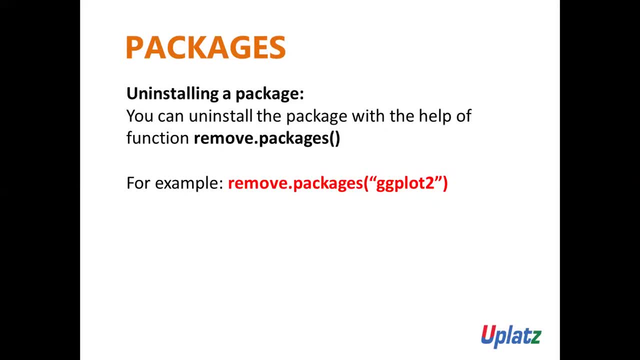 So with the help of function removepackages, Okay, So with the help of function removepackages, and then specify the name of package that you want to remove, like this, you can easily uninstall the package. Okay, Now let me show you next thing. 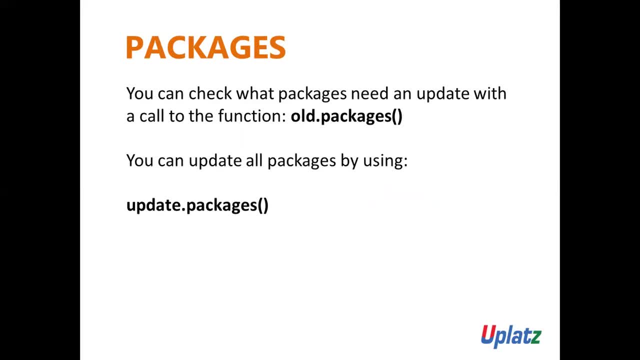 You can check what packages need an update with a call to the function oldpackages. Are you getting it? You can check what packages need an update with a call to the function oldpackages. Okay, So this means, with the help of function oldpackages, you can check what packages needed the update. 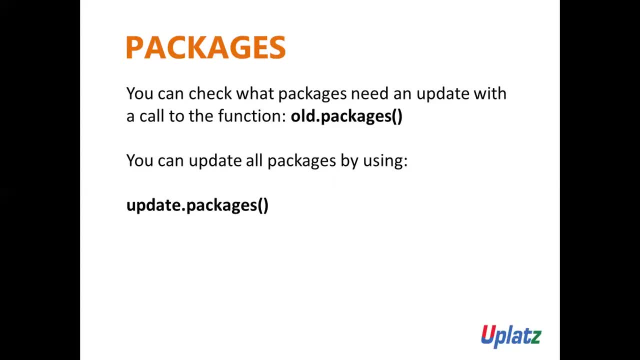 Got it And then, in order to do the update, okay, For all packages, there is a function updatepackages. So, with the help of this function updatepackages, you can update all the packages And with the help of function oldpackages, you will come to know what are the packages. 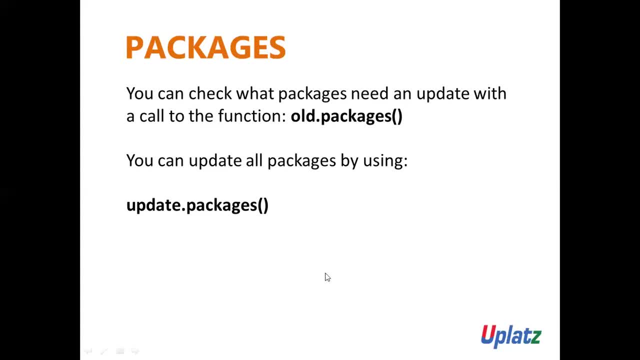 that required the update. that need the update. Okay, Got it. So oldpackages: that will show you what packages need the update and updatepackages means you are going to update all the packages. Now let's see unload the package. 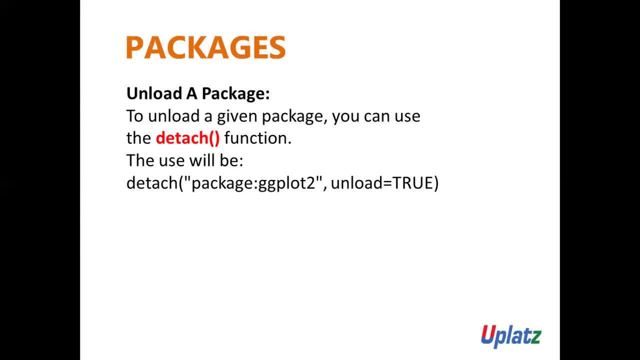 See here we have seen how to install the package ggplot2 with the help of function installpackages inside the opening closing bracket double quotation: ggplot2. and in order to use this package, We have used the library function ggplot2.. In order to use it, we need to load it with the help of library inside that we need to. 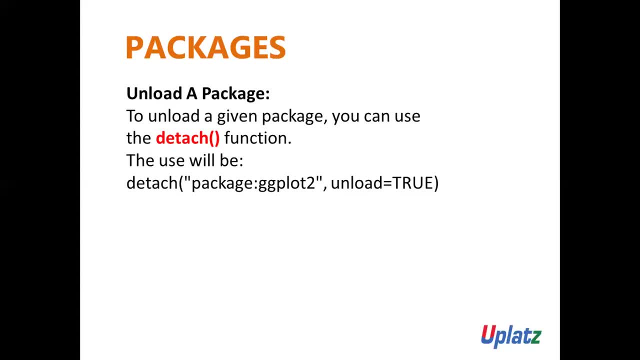 specify the name of the package that we want to use. Okay, Now next thing is to unload the package. You can use the detach function, For example. the use will be detached: package, For example: in our case, what is the package you want to unload? package colon: ggplot2 unload. 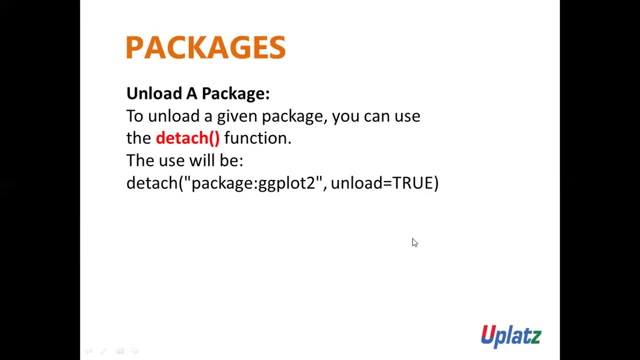 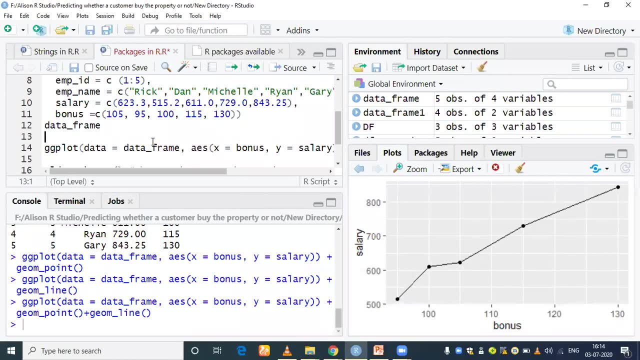 is equal to true. like that We need to use. like this. Got it Now let me show you all these details in R studio. So I have opened R studio. So we have seen how to plot, how to make a plot with the help of ggplot2.. 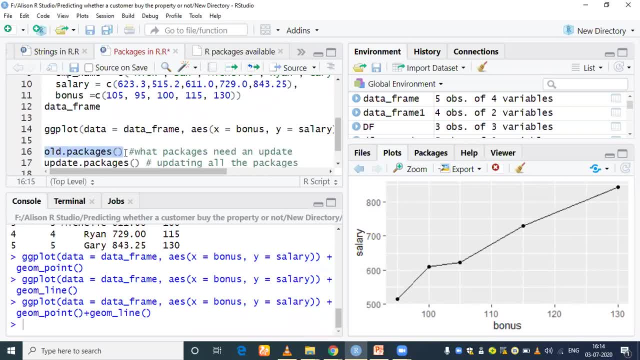 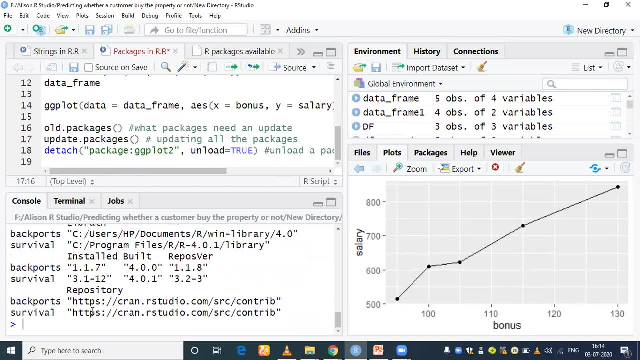 Now, what is this? oldpackages? It is going to see what packages need an update, So let me execute line number 16.. So see, wait a second. Can you see the output? now, After executing line number 16,, I'm getting this output. 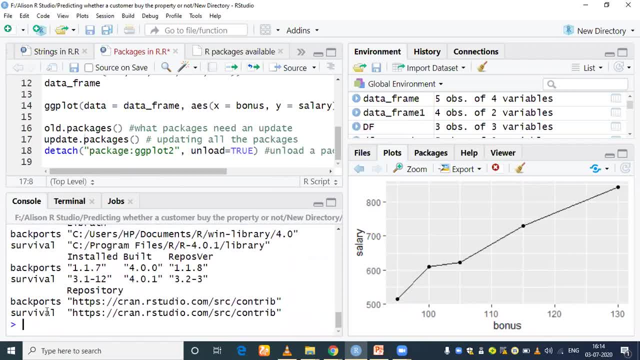 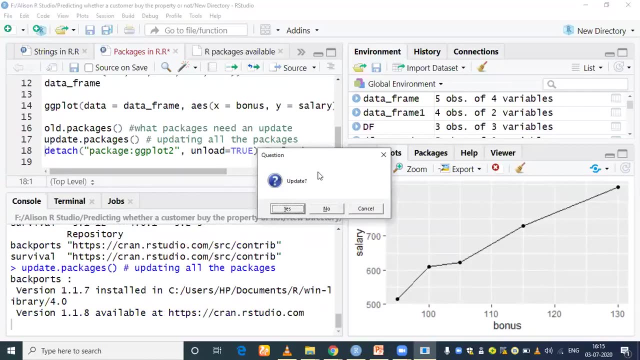 So these are the packages that need an update now. Now update the packages. If I execute this line, it is going to update all the packages, am I right? So let me execute line number 17 and let's wait for it. Yeah, the question is coming here: update yes or no? 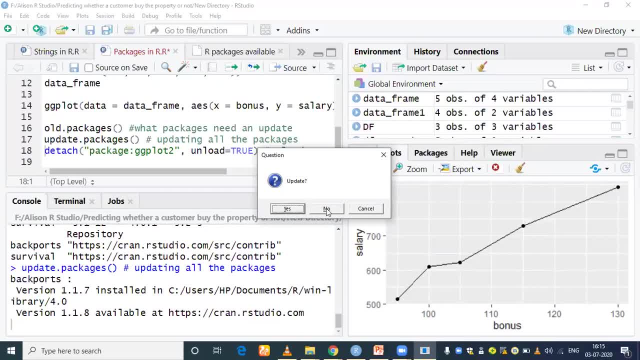 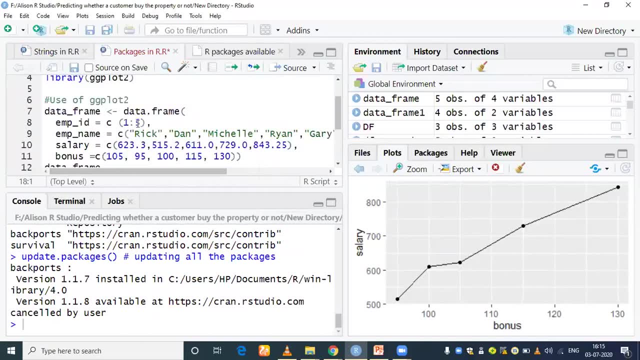 So if you want to update it, you just need to click yes, otherwise no, got it. Now. next thing is how to unload the packets. Currently we have load the package. What package? ggplot2 with alpha function library. Okay, 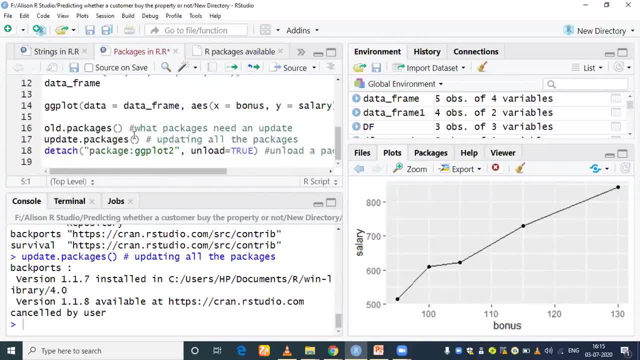 Now, in order to unload this package, I need to use the function detach. Okay, So detach package. colon: name of the package that you want to unload. command unload is equal to true. What is this? It is going to unload a package. 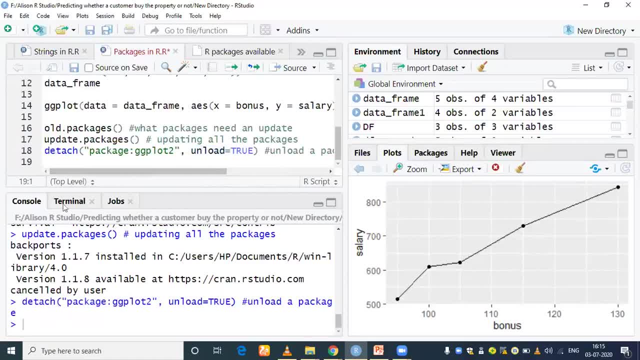 So let me execute line number 18.. So see here, line number 18 has executed successfully. This means currently we are just unload the package with package ggplot2.. We have not removed it, Am I right? Does we remove the package ggplot2?? 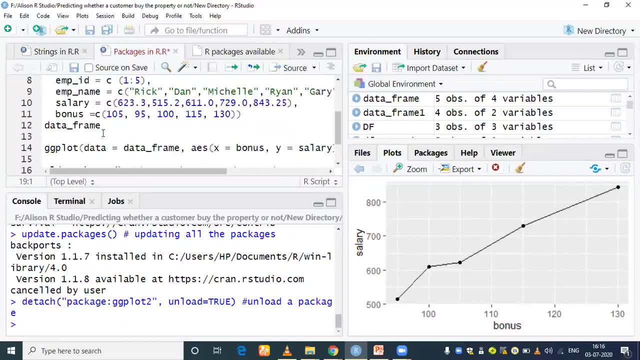 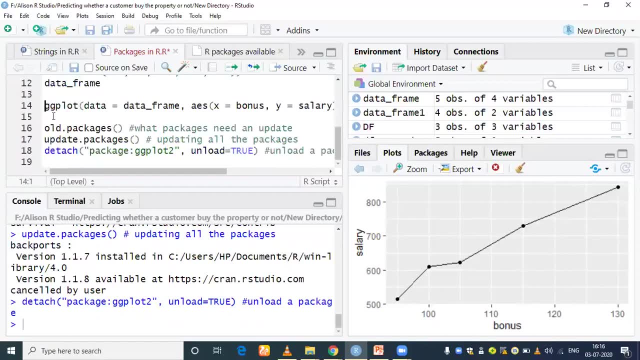 No, we will just unload it. Now. if I execute this line, which line? ggplot? ggplot is a function which is present inside the package ggplot2.. If I execute line number 14, can you see that I'm getting the error? 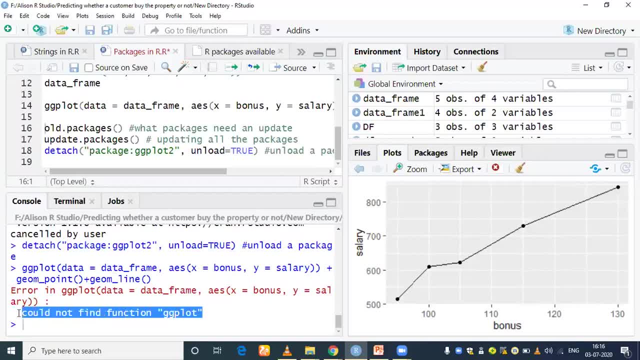 Could not find the function ggplot2.. Why am I getting this error? Because I have unload the package ggplot2.. Are you getting it Now? if I want to use it, First of all I need to install the package ggplot2.. 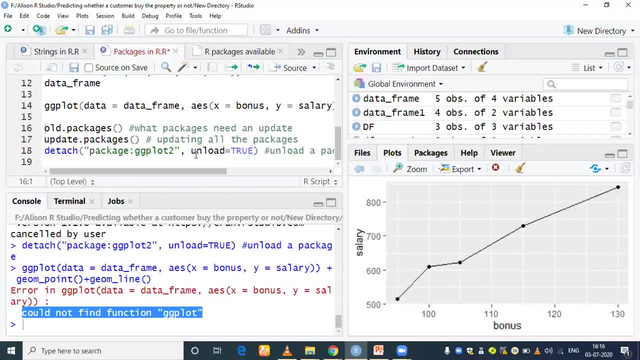 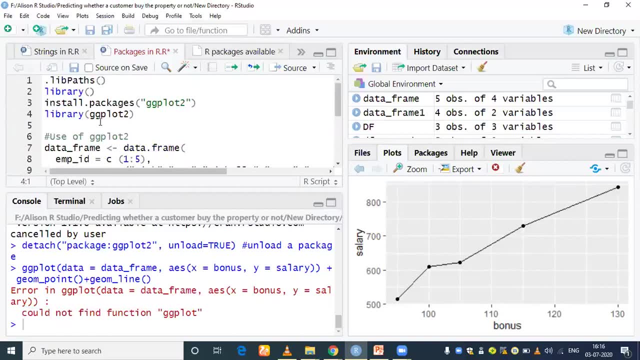 all i need to install the package. so i already have installed the package ggplot2. in order to use it, i just need to load it with the alpha function library ggplot2. so if i execute now line number four, can you see that warning message? package ggplot2 was built in under. 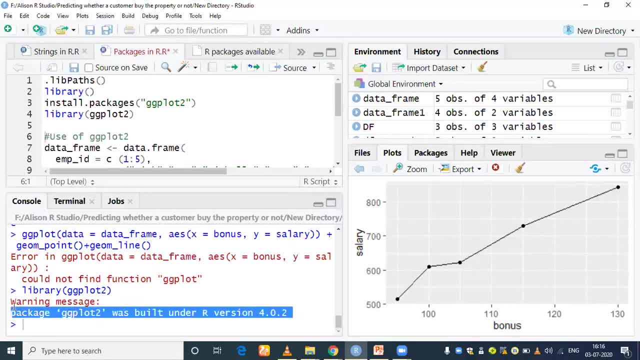 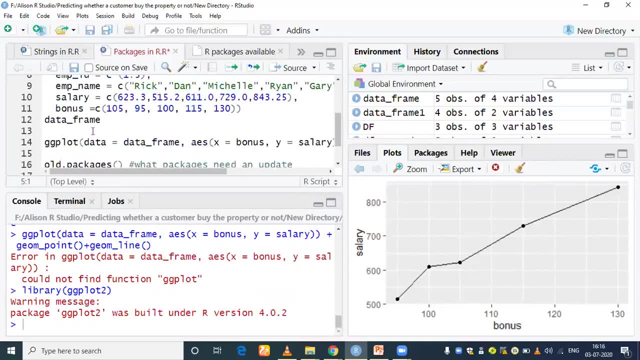 see, it's a way, just a warning method. it's not a error. so this means now we can use: after executing line number four: we have loaded the package ggplot2. now at this time, if i execute line number 14, can you see that output is coming here, the plot you can see on the right side. 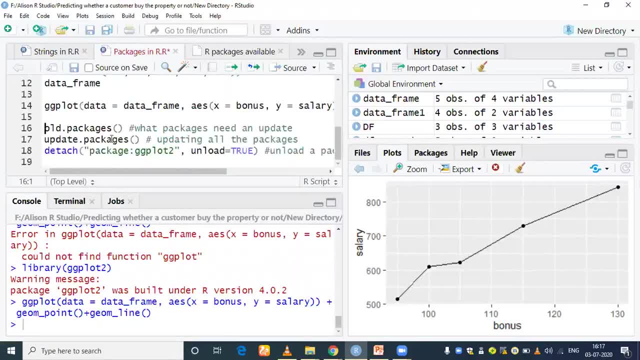 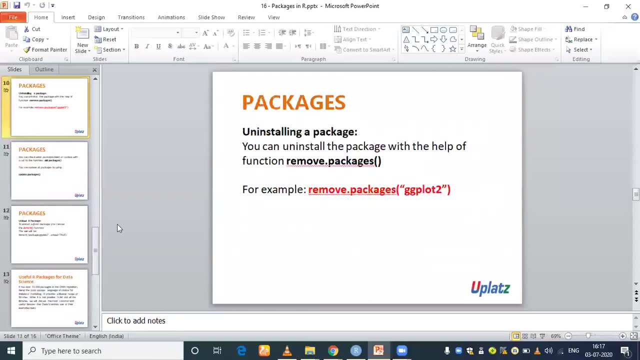 so this means it's loaded. now again, if you want to remove the loaded package- this one- you need to use the line number 18. got it now. next thing is how to uninstall the package. yeah, how to install the package with the help of function remove dot uninstall. sorry, remove dot packages. 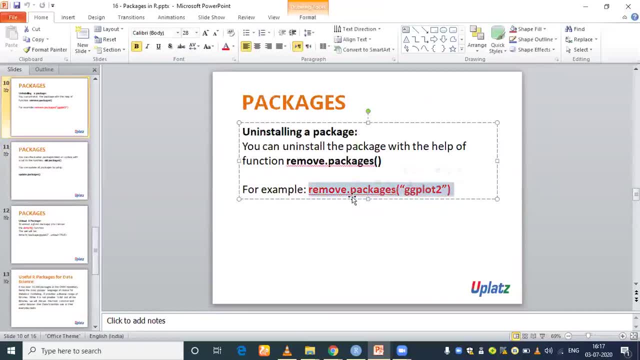 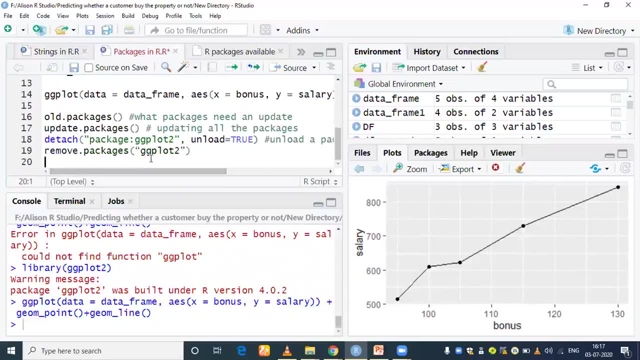 see here: if you write this, remove the packages, you are going to uninstall the package. okay, so i will write this line here. see here: remove dot package, the name of the package that you need to uninstall. so what is this? it is uninstalling. it is going to uninstall ggplot2 package. 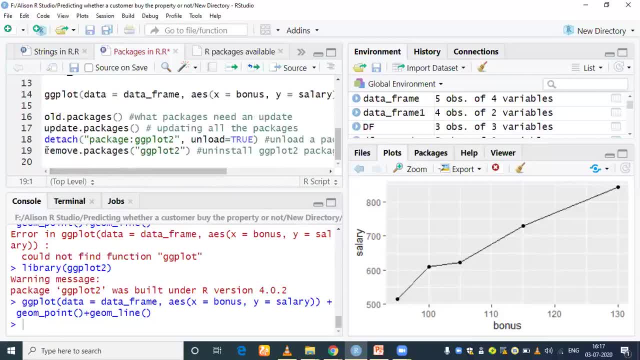 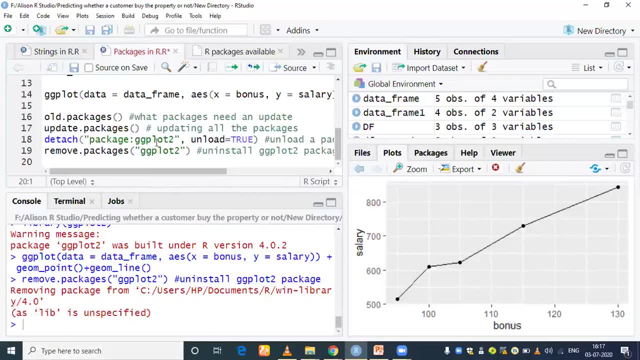 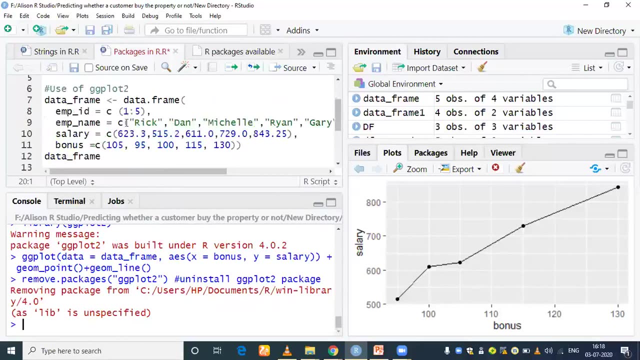 got it. so let me execute this line, line number 19.. see, here it's coming, removing package from this one. got it now. let's check it now if you want to again use it. library ggplot2. so see, after installing the package ggplot2, you can. 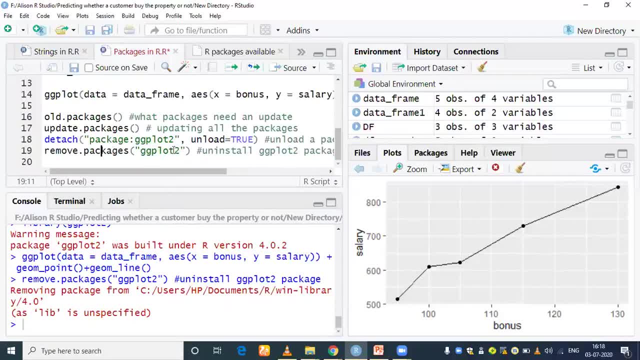 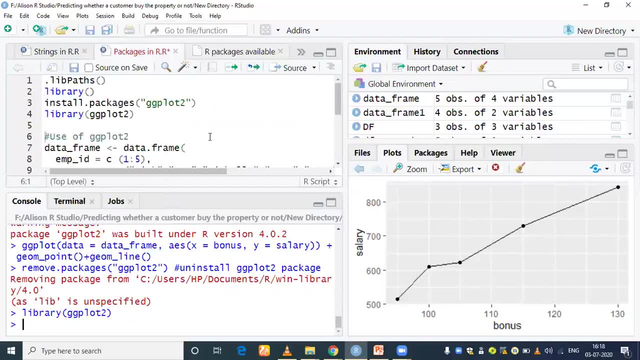 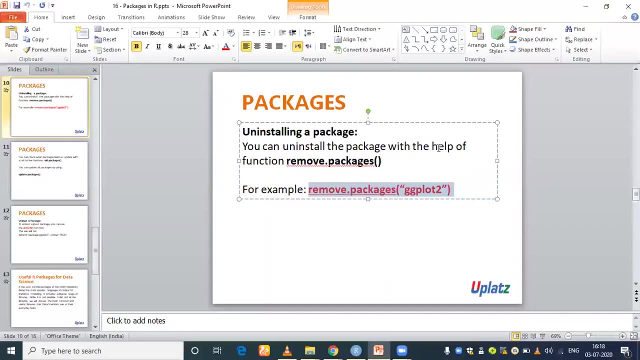 load it. now what i have done. i have removed the package ggplot2. now, if i execute line number 4, see here it's now loaded. got it, so see here: remove that packages. what does it doing? you can install the package with the help of function remove dot packages. 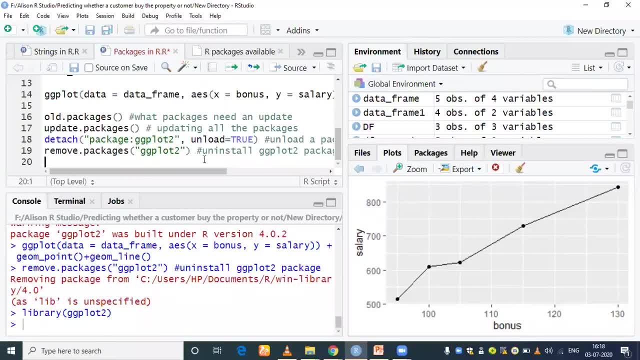 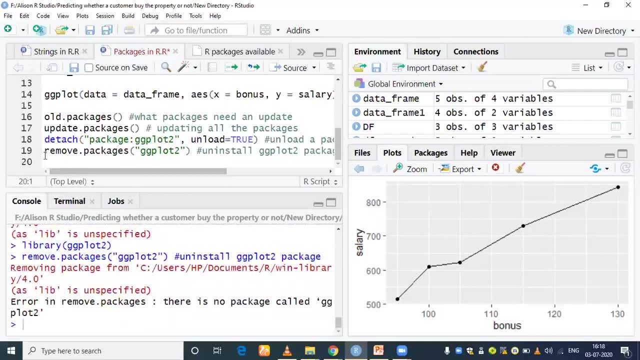 and then specify the name of the package. see here again what i have done. i executed this line two times. am i right line number 19? now, at this time i'm getting the error. error in remove dot package. there is a no package called ggplot2 can. 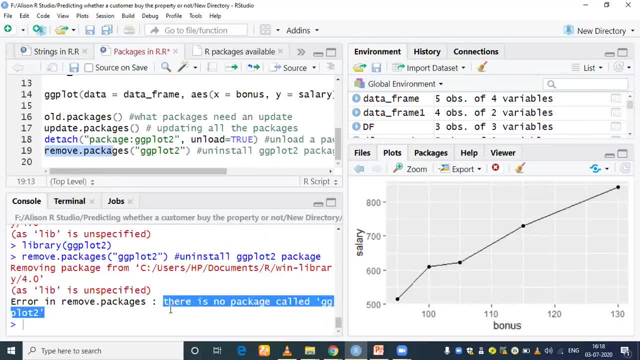 you see this one. there is a no package called ggplot2 got it. this means we have successfully removed the package. ggplot2 got it. so to remove the package or to uninstall the package, we need to use the function remove dot packages instead that we need to specify the name of the package that you want to. 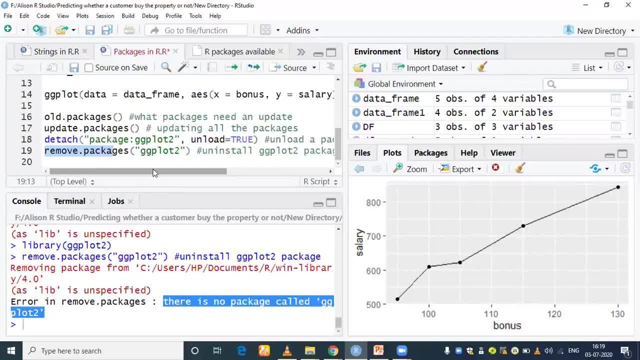 uninstall or that you want to remove. so see, here we are getting the error. if i execute again line number 19, so i'm getting the error here. let me again execute it. can you see the output here? error in remove dot packages. there is a no package called ggplot2 got it. so now we have seen. 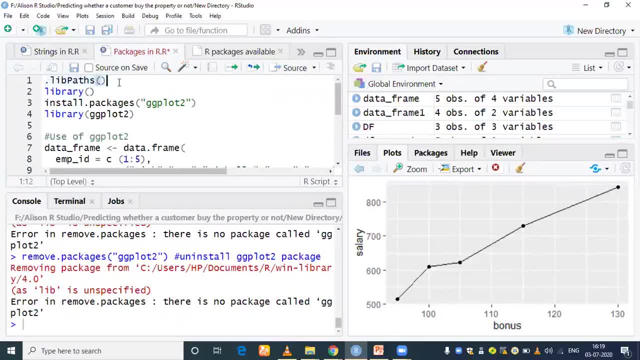 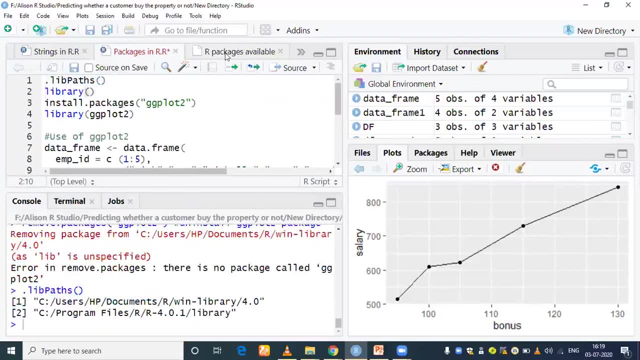 with the help of dot lib, it is going to show us where. what is the library location. okay, this is our library location where the package is installed. with the help of this function library, we can see the are available packages. there are packages available in the directory and then, with the help of installer packages, if you know the package name, you're. 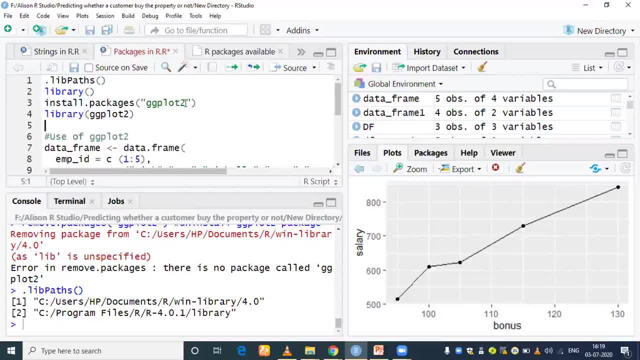 going to install the package. after that, you're going to install the package. after that, you're going to install it. ok, so now this is the ggplot2. in order to use this package, i need to use, i need to load them with the help of function library. okay, and inside there i need to pass the name of. 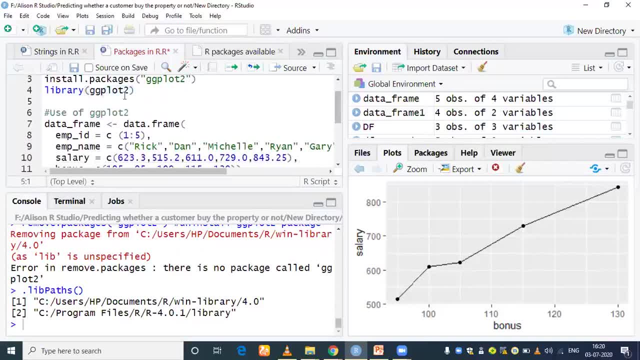 the package and then after that, we have seen: in order to use the function ggplot2, which is present inside the package ggplot, uh, in order to use the function ggplot, okay, we have loaded ggplot2 package and then we have created a data frame, okay, so that we can use it inside our function ggplot. 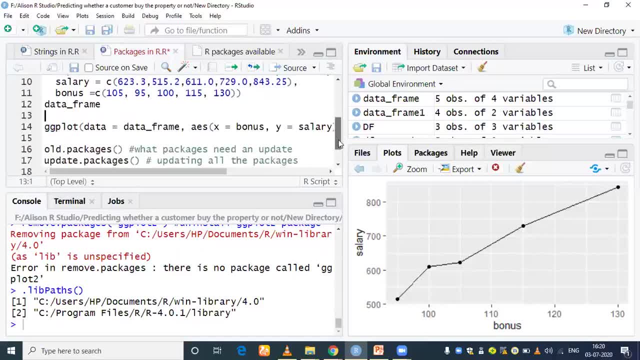 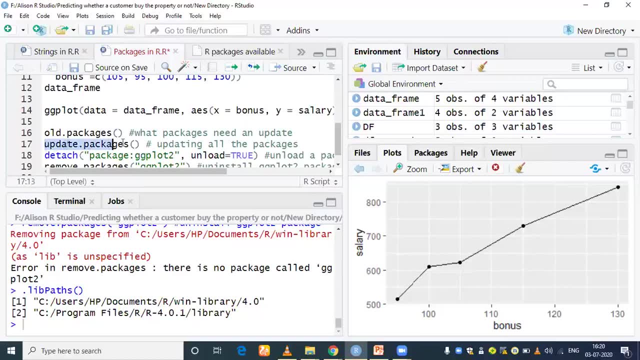 package, ggplot2 got it, and then we have seen what packages need an update. how can you take it? with the help of all dot packages- and if you write update dot packages it is going to update all the packages- and then, with the help of detach, okay, this function. it is going to this line of. 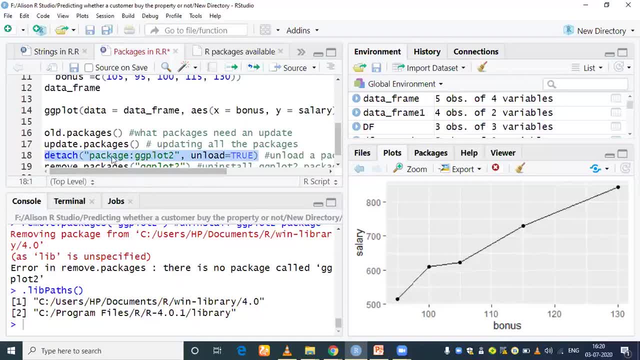 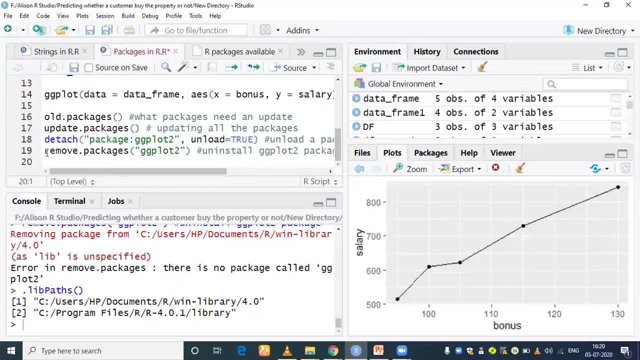 code. it is going to unload a package, so package colon, name of the package. comma unload is equal to. and. finally, in order to uninstall the package, there is a command. result function for us remove dot packages is to write the name of the package. got it? yes, i hope you understand now. now next. 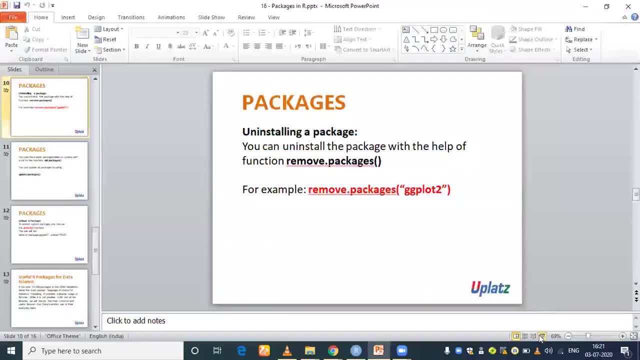 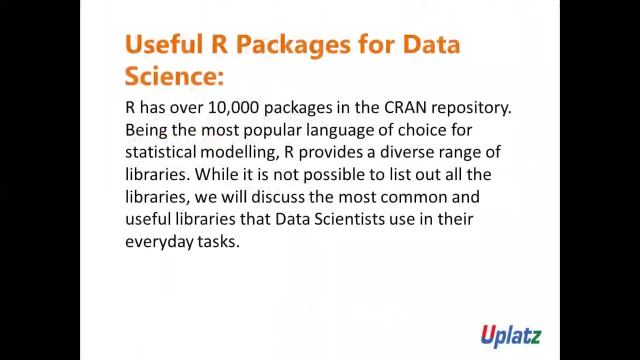 thing. let's see the next thing about package. so we have seen detach function. okay, now let's see the useful r packages for data science. r has over ten thousand packages in c, r, a and cran repository, yeah, being the most popular language of choice for statistical modeling. r provides a diverse range of libraries. while it is not possible to list out. 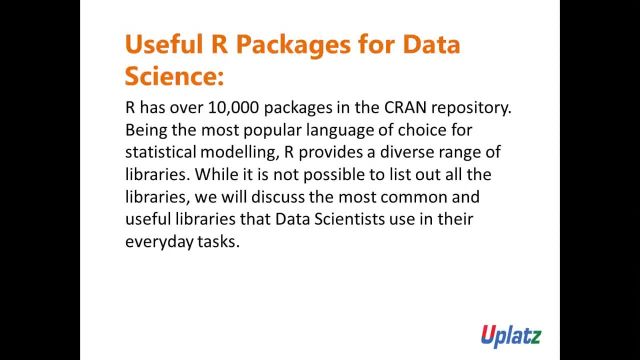 all the libraries. we will discuss the most common and useful libraries that data scientists use in their everyday tasks. okay, so if you would like to become data scientists with the help of r, you should need to know what the libraries they are using nowadays in everyday tasks. yeah, so let me show you that. 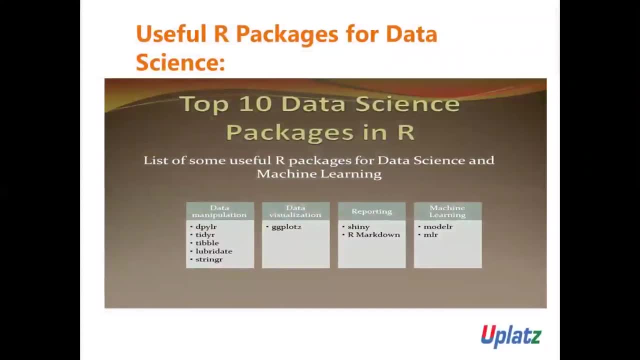 so see here useful r packages for data science. top 10 data science packages in r. okay, top 10 data science packages in r. so i have just written the top 10 packages. so list of some useful r packages for data science and machine learning. so see here for data manipulation: data. 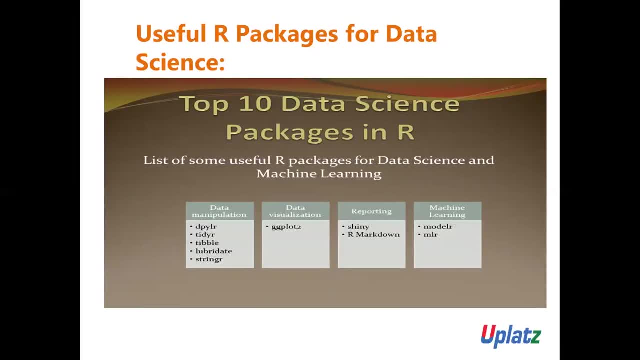 scientists are now using the packages name, depler, tdr, table okay, lubricate and string r for data visualization. the most useful package is ggplot2. yeah, we have seen the example of ggplot2. how to install this package, how to load this packet, how to plot, how to make a plot with 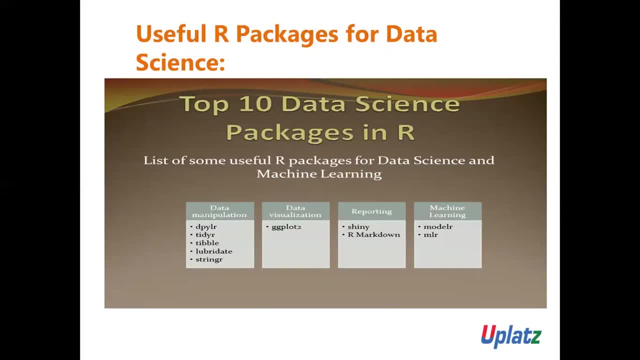 the help of ggplot function. yeah, and for a reporting- shiny shiny is one of the packets- and then r markdown. and for a machine learning, they are using the package model r and mlr. got it? yeah, these are the some important packages nowadays that the data scientists are using okay.